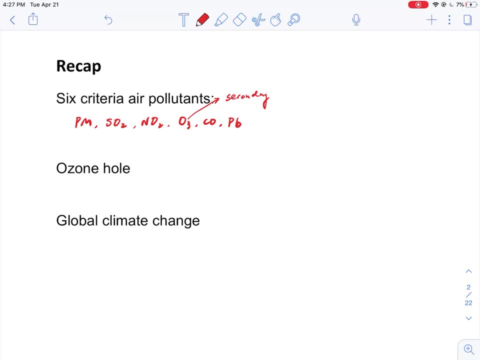 mainly because it's not directly formed from emission sources, but it's formed based on existing air pollutants, right, And for all the other five they are primary air pollutants. So we further introduced the ozone hole right. So that's the stratospheric ozone that's forming. 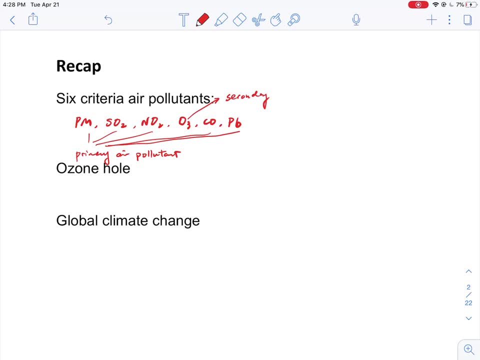 a layer of air that's protecting us from the UV radiation, right. So we mentioned that the ozone hole is mainly because of people emitting the CFCs- chloroplasts, Right, And the CFCs, although they're very stable in the troposphere, right in our atmosphere. 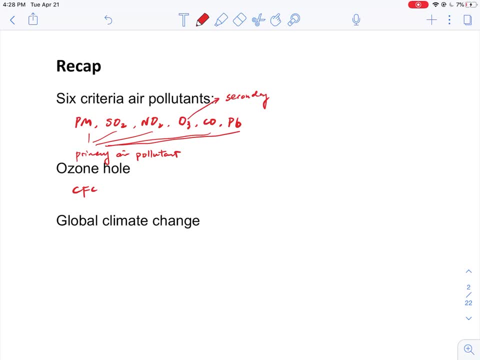 but once they get leaked into the stratosphere they're a catalyst right, So they can destroy the ozone with an infinitely long time And it's very difficult to degrade or to remove the CFC. So also mentioned about the global climate change right, So we saw that there is really 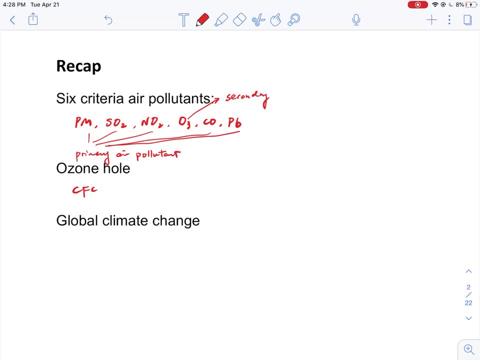 a long way for people to go to solve this issue here. So in this class we're going to focus on one type of the six criteria- air pollutants- And in our next class we're going to talk about the remaining five right or some of them, which are the gas or the gaseous air pollutants. 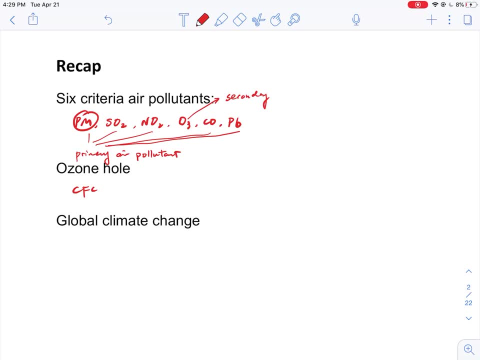 So the particulate matter are basically particles suspended in the air, right? So according to a more specific definition or more complete definition, PM is defined as a stable cluster of molecules, right? So as long as the molecules form a cluster and they're stable enough, then we can call them as a particle. So let's think of nitrogen. 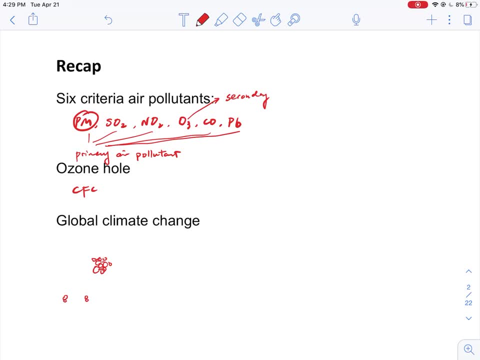 right, So we know that nitrogen is composed of two nitrogen atoms. right, This is nitrogen molecule, So a nitrogen molecule itself. right, so we define that PM is stable cluster of molecules, So only one molecule. So one molecule doesn't qualify as a particle, right? So once they collide each other, we know that they. 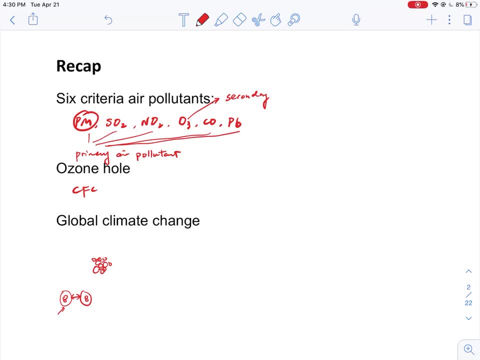 are very unstable, right? So as soon as they collide to each other they'll disassemble, right? So a cluster of nitrogen molecules cannot count as particles, right? So let's see if we have a bunch of, for example, water molecules, right, if the temperature is right enough, or if we have a 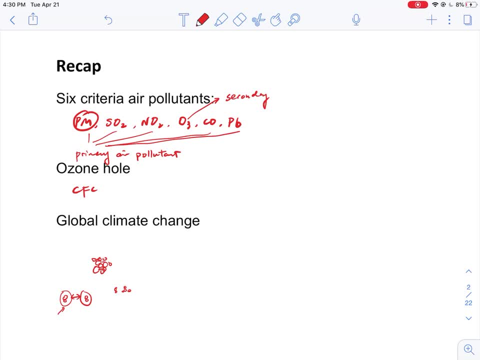 high relative humidity, then we. so an example is during the winter, when we try to exhale the air from our mouth. no, then we can typically see smoke, right, see like a hazy water droplets in front of us. so those water droplets are stable clusters of molecules. right, because they form large enough. 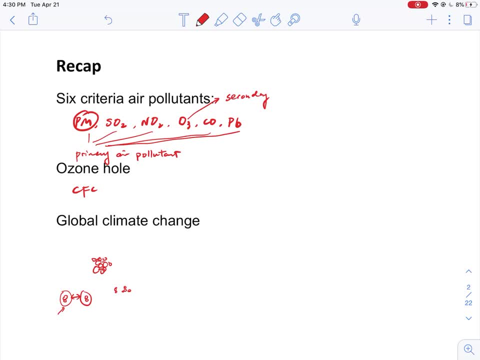 particles that are stable, that existing in the atmosphere, right, so those are called particles. so if we further expand the definition of this pm, so let's think if is our earth a particular matter? it is right, the earth is very stable and it's also a cluster of molecules. because of that, 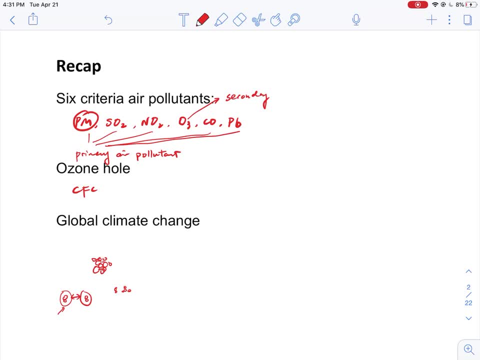 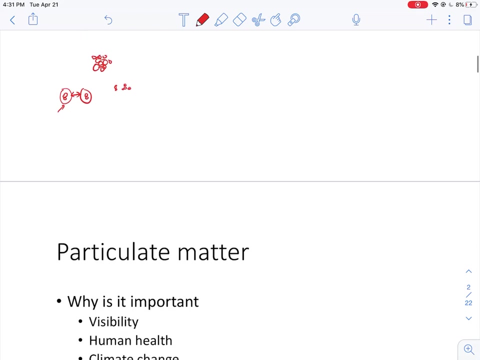 a football is a particular matter. a potato is also a particular matter, right? so this is in terms of the broader definition of particular matter. but here we're just treating this particular matter as something that's suspended in the air, right? so we can further go through this definition at the end of our class, right? so we talked about particular. 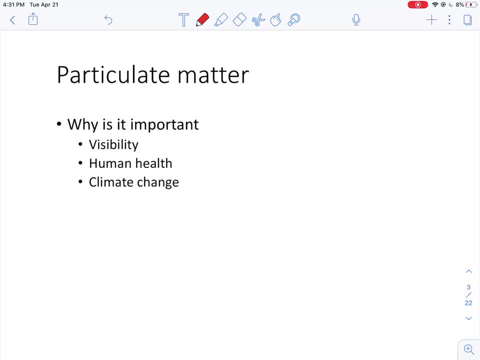 matter quite a lot, right. it's also one of the six criteria- are pollutant. so why is it very important? so why is it important, right? so, of course, the perigee matter can affect the visibility, so I'm sure that you have heard of the great smoke. 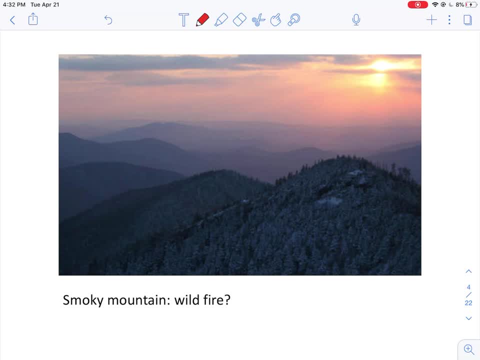 mountain. probably some of you have already been there, so the smoking mountain are actually famous for its smoky or hazy feature, right so, just as shown in this picture here. so we are seeing this layer of smoky air there, right so this smoky feature is actually because of these suspended 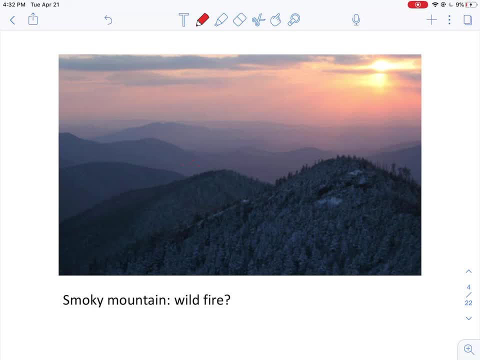 particles, or particularly matter in the air. so then you may wonder: where are these particles coming from, right? is it because someone barbecuing in the water, in the, in the forest? i don't think that they have so many campgrounds all over everywhere, right? so the reason why we see these particles is actually because, um, because, on one hand, forest, 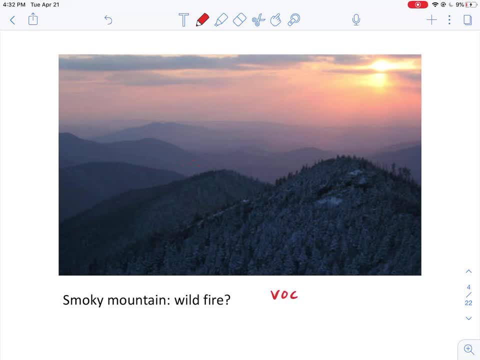 forests themselves emit a lot of volatile organic compounds, which are the organics, right. so we have a lot of pine tree, we have a lot of other type of trees, so they will emit those gaseous species into the atmosphere. well, at the same time, we know that smoky mountain is. 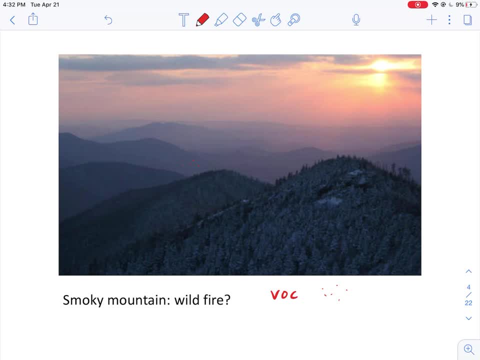 close to atlanta, so atlanta have a lot of industrial facilities there. so the industrial facility will emit nitrogen oxides and sulfur oxides. so once they mix together they are going to form stable clusters of molecules, and also the solar radiation will also promote this particle. 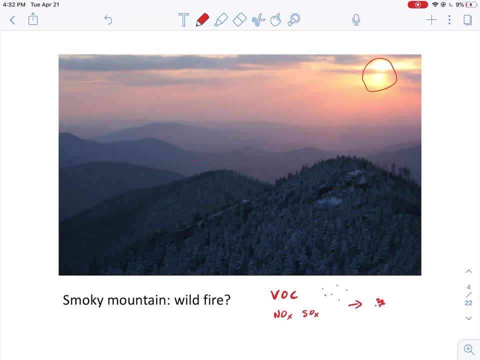 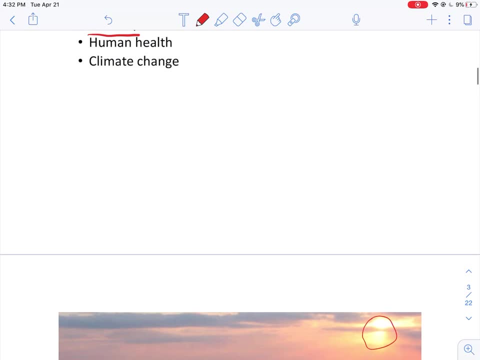 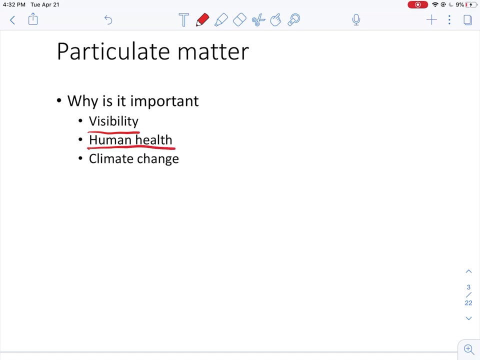 so we're able to form those larger particles and it's giving the forest or giving the park a hazy feature there, right so the pm can affect the visibility. so also pm will also strongly affect the human health, because we mentioned that particular matter is very harmful to people with. 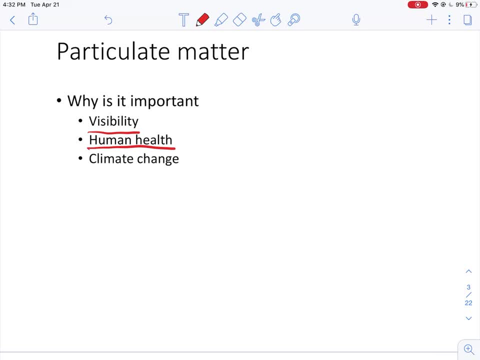 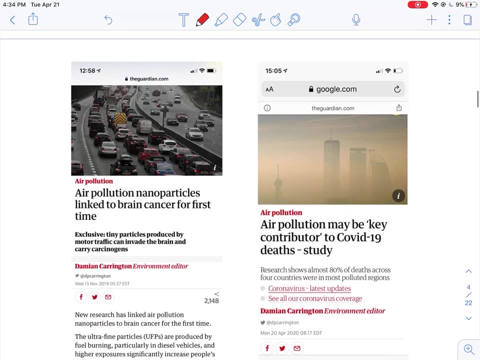 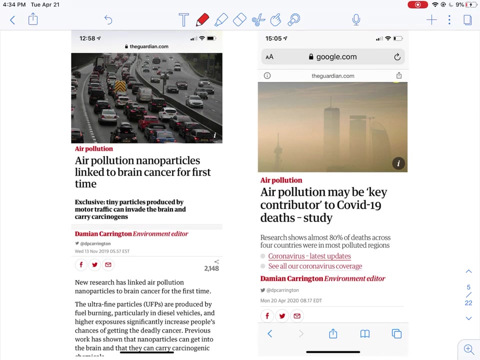 respiratory diseases, right. so once they get into our respiratory system, they can cause allergies and all different types of diseases. and actually it was until recently. you can see that this article on the left from the guardian right so that was published uh 2019 in november, right it? 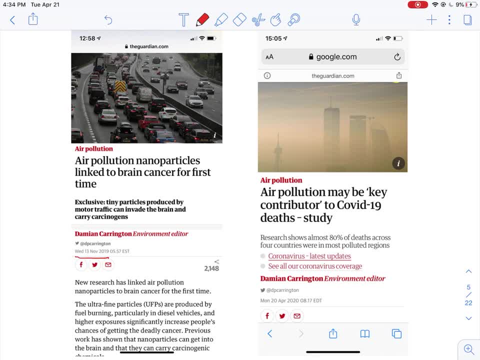 is until recently that people started to build a relationship between the air pollution, nanoparticles and the brain cancer. okay, so the higher the concentration of these air pollutants, or pm, the susceptibility or the probability of people getting brain cancer there. so, uh, also recently, it's actually these days. so the scientists are also seeing that the air pollution might be a. 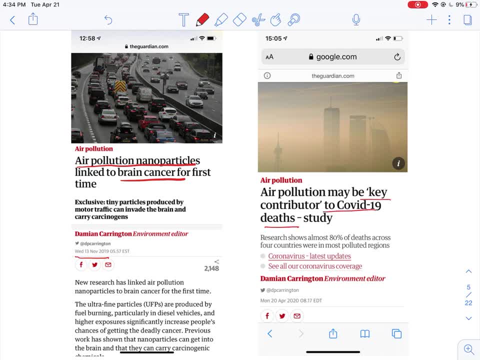 key contributor to the covet 19 death. okay, so people analyze quite a lot of data right to analyze the mortality rate of the covet 19 and then found that they actually can correlate well with air pollution. so for this study there's also a lot of controversy because 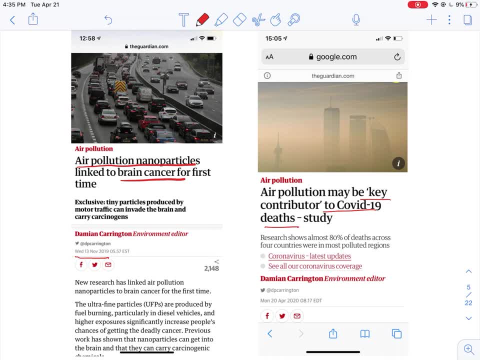 if you think about the mortality rate of copy 19, so it is first or directly related with what is a vacancy of the icu beds. so if there's not, if there's not enough icu beds, then the mortality rate will be very high. but on the other hand the icu bad number is somehow related. 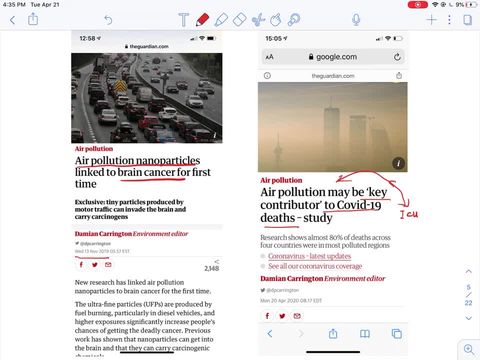 with the air pollution because they may be related with poverty of that specific area, right? and then further get involved in the air pollution. so of course, a lot of more studies are still needed, right? so on the other hand, people were saying that it's probably because the air 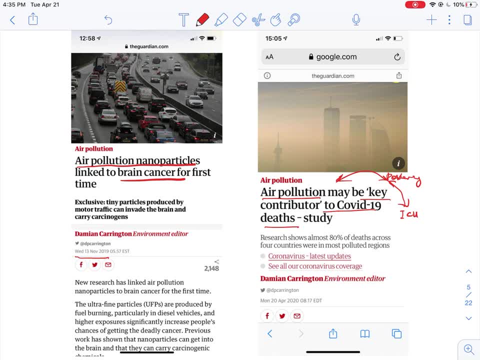 pollution caused some lung diseases for those patients and further increase their mortality. but until now, i don't think there are studies looking at each patient and see what is their existing diseases, because existing diseases not only includes respiratory diseases, they also, you include diabetes or high blood pressure, so on, right. so of course, a lot of more studies are. 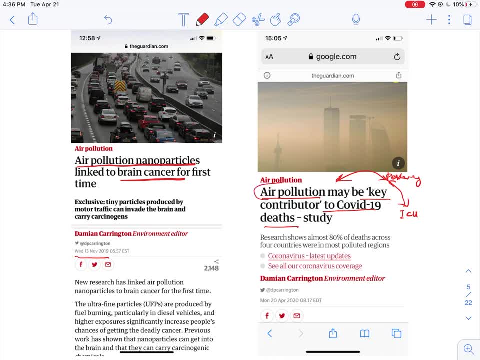 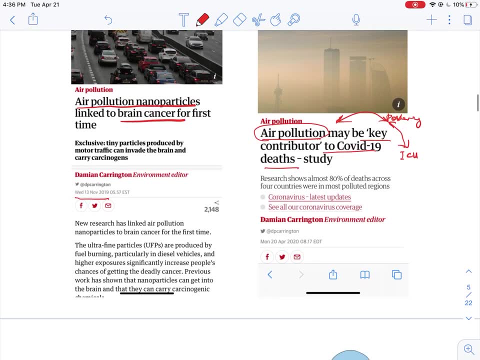 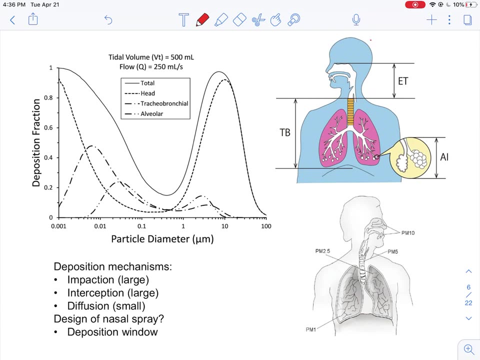 needed, but it's good that people are starting to notice that air pollution can actually lead to quite many consequences. okay, and further in terms of the health aspect of the particular matter. so here what i'm showing is that we can actually divide our respiratory system to different regions. 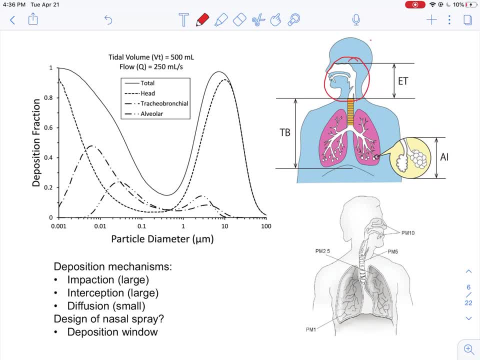 right. so there's a region called the head region or the external region right, and then we have the tracheobronchial- which are these branches here- or the tb region, and then finally we have this really deep lung region or deep pulmonary region, that's called the alveolar region. 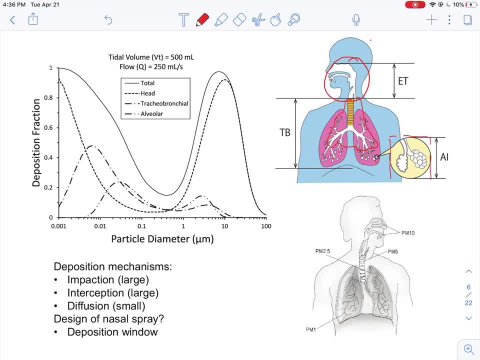 right, so these are the region where the oxygen will exchange, or the red blood cell will exchange the oxygen with carbon dioxide, right so as for the particular matter, so once they get, or once they get inhaled into our human body, they can get deposited in different regions. 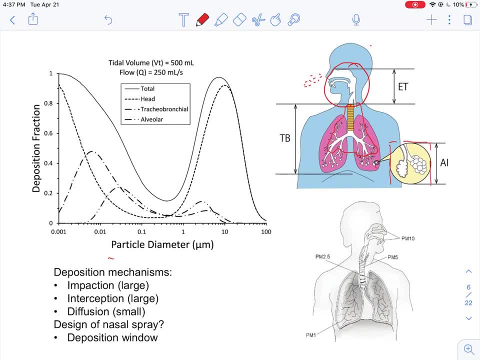 and their deposition fraction is a function of particle diameter. it depends on their size. so you can think that actually for smaller particles they can penetrate further into our lung, right? so there's a higher probability that they may be further get deposited into our deeper respiratory system. but at the same time, for the smaller particles, because they have a 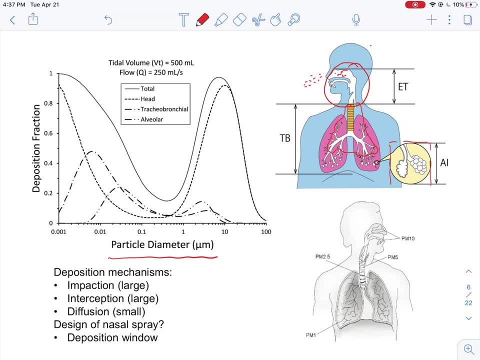 high mobility there, so there's also a higher fraction of them getting into our head airways. so here you can actually see how for how, basically how different areas of the respiratory system will respond or can collect these particles with different sizes. let's say, for example, we're talking about the tracheobronchial region or the tb region, where there's a lot of tubes. 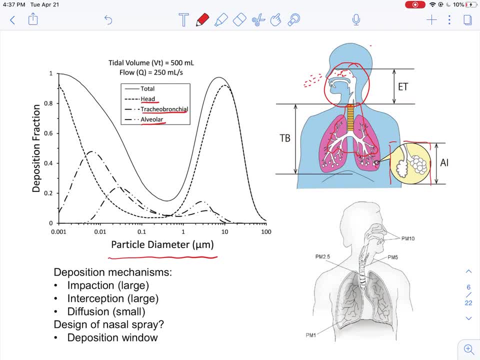 right. so for the tracheobronchial region, then they will represent basically this part. they will represent this part. so one line and two dots, right. so what this simply means is that for tracheobronchial region they will have a and further, for 20 nanometer particles, this is 0.01, 0.02. 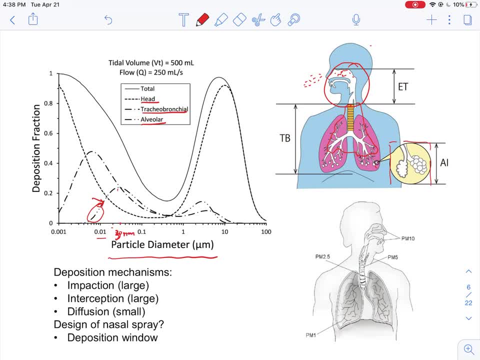 30, actually 30- nanometer particles. they will have a and around 22 percent getting deposited into the tracheobronchial region, while for the head airway, we're looking at maybe around 10 percent of them getting deposited into the head region. 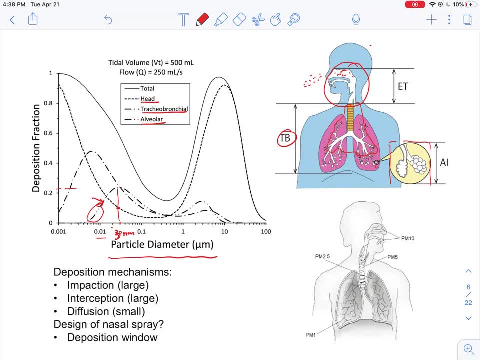 right. so basically we can sum up of all of these different uh deposition efficiencies and then come up with this solid curve here. so basically this curve represents how our respiratory system can collect these particles and search if they might be before they even deeply, with different sizes, And, of course, if these particles carry viruses, for example the SARS-CoV-2. 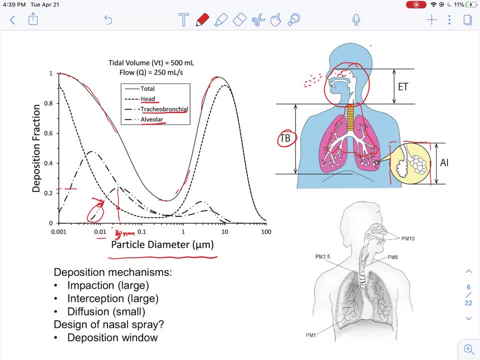 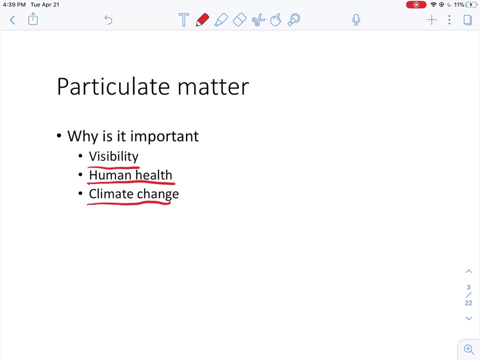 virus, then they can further get penetrated into our body and then transmit the disease to human right. So we'll further talk about this later. And finally, the particular matter is also important because it's until recently that people realized this PM can cause global climate. 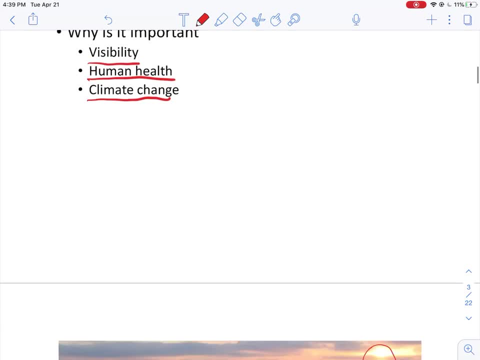 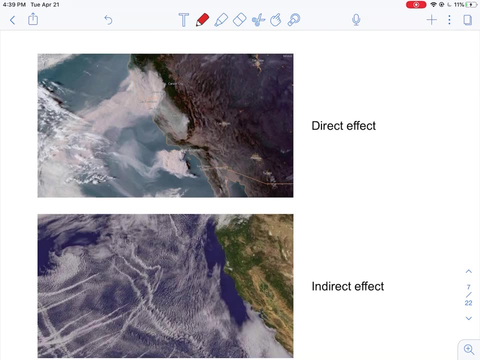 change. So you may think: why is it related to the climate, right? Why is it related to the temperature of the Earth? So, if you think of the situation, let's say: this is our Earth, right? And basically, if we cover it with a layer of white clouds, what's going to happen? Okay, 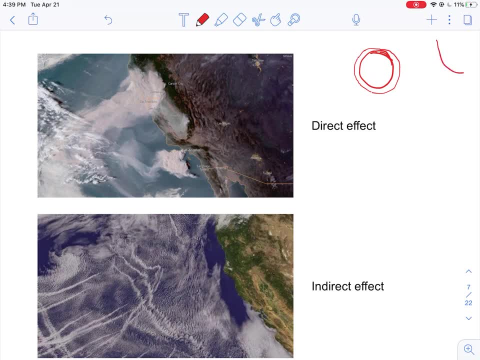 so what's going to happen? What's going to happen is, let's say, this is our sun, and then the sun is emitting different radiation into the Earth, right, And that's the source of the heat actually on our Earth. 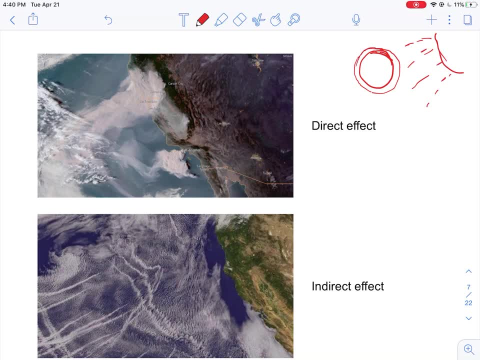 So if it's covered by a layer of clouds, because the cloud is so white. so basically, these radiation will get reflected into the universe. So there's no way that the radiation, or only a small fraction of the radiation, can penetrate through the cloud and then heat up the Earth, right? So 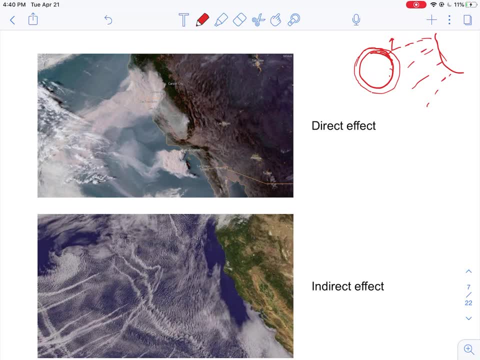 basically, people call this as a snowball effect. right, We form a layer of cloud and then that's going to reflect all the radiation back into the universe. And actually, what's keeping our Earth warm is because of these oceans, these darker regions, which absorb this radiation and warm up the Earth. 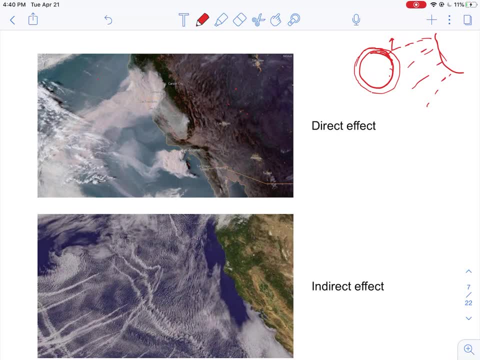 okay. So this simply means that the more cloud, then the more cooler, or the cooler the Earth is right. So this is how the PM can get into the picture. Let's say, recently we had quite a lot of wildfires, right? So first it's in California. 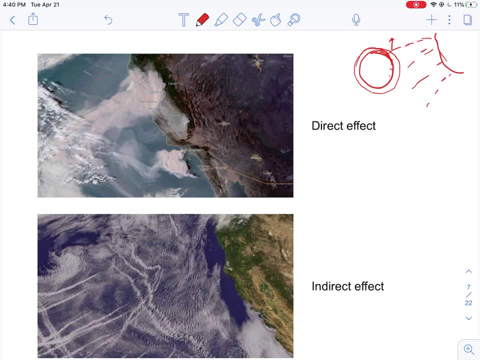 and then in Australia. Australia had a very long period of wildfires, So these wildfires emit a lot of smoke into the atmosphere, right? So this is the satellite image of the California coastal region, right? So you can see that the wildfire generates a lot of these smokes here and the smoke look 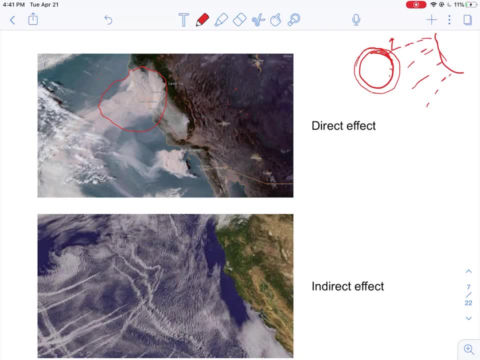 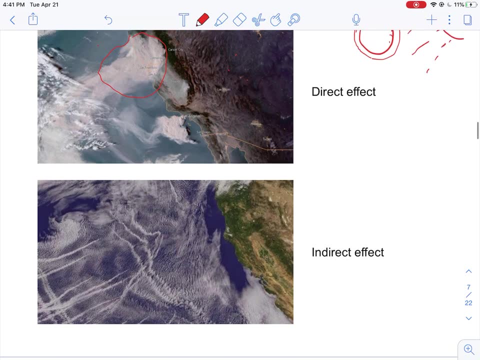 white. right Because of that, the smoke looks white and the smoke looks white and the smoke looks black. right Because of that, the radiation will get reflected into the atmosphere and actually it's causing a net cooling effect on the Earth. And, furthermore, what we can see is that these 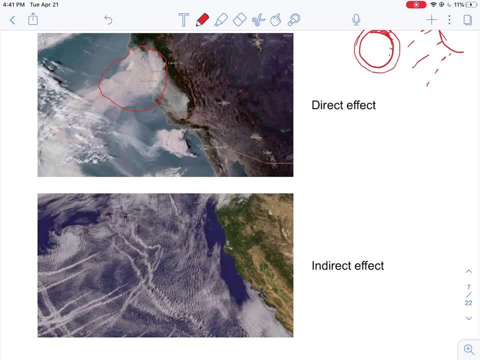 particles can actually further form clouds. So not only there are smokes, but each single of these particles here can further absorb water and then form cloud droplets. So for example, these here: you can still see them behaving as smokes here, But let's say here: 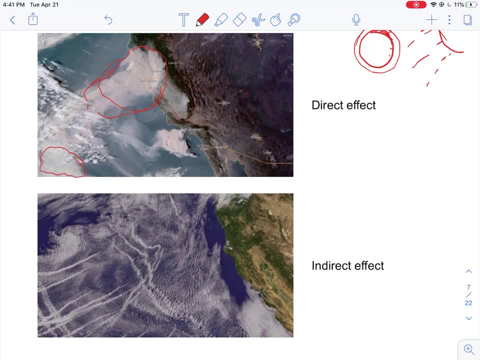 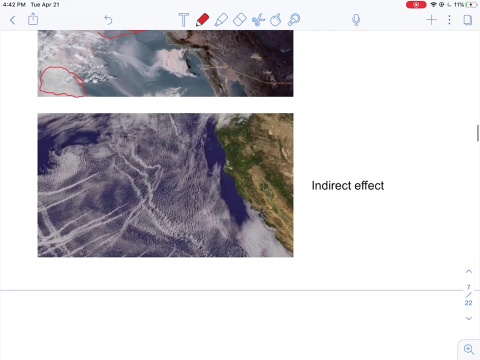 the smoke can absorb enough of water over the ocean and then further expand in their size and then further form the clouds. So you may see that, oh wow, this doesn't look very direct or straightforward, right? So let's look at the second picture. So, again, this is a picture of the 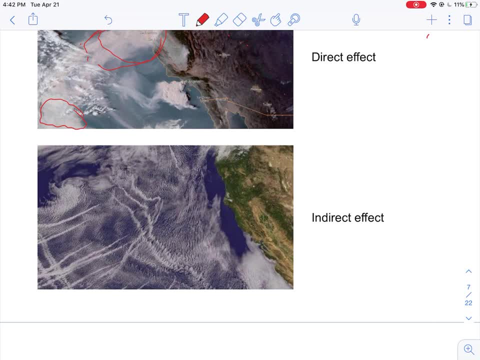 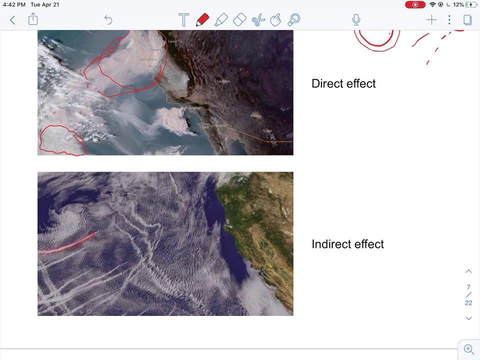 California coast region and you can see there are a lot of clouds over the ocean, right, But among these clouds, you can see these very thick clouds, and you can see these very thick clouds and you thin clouds here, right, they exist in the form of stripes. so what are they actually? these are ship. 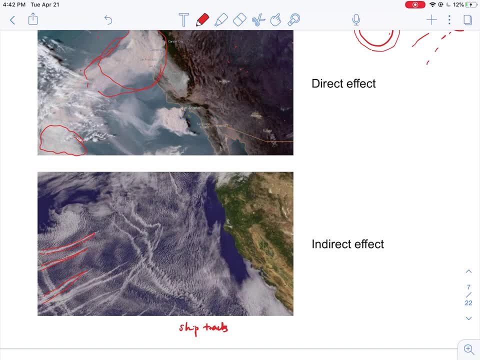 tracks. so basically, the ship will go from one point to the other location, right. so at the same time they will emit particular matter into the atmosphere and as they further travel upward they can absorb enough moisture and then form the cloud droplets. and once they form the cloud droplets, you. 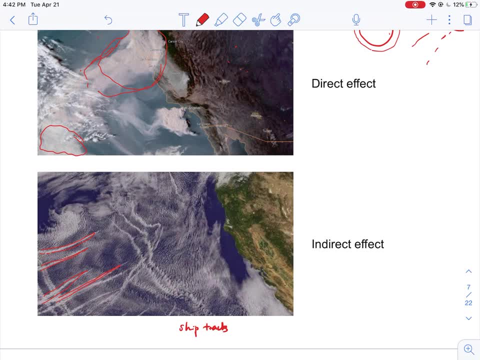 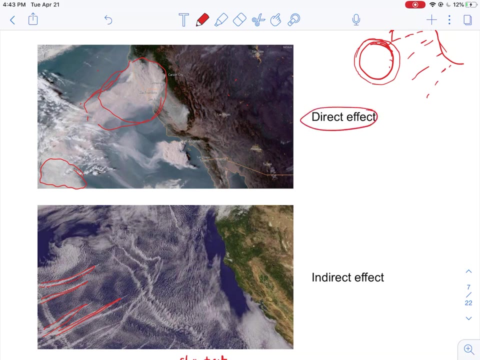 can see these really long stripes of clouds, and this is a direct evidence of how the particular matter can affect the cloud formation and further affect the global climate. so you can see that the climate impact of the particular matter can exist in two ways. one is the direct impact: right, so we're forming smoke that can reflect the light, and there is 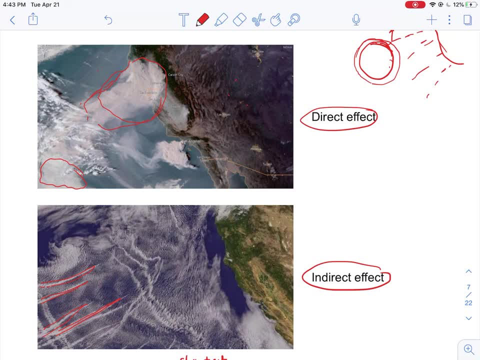 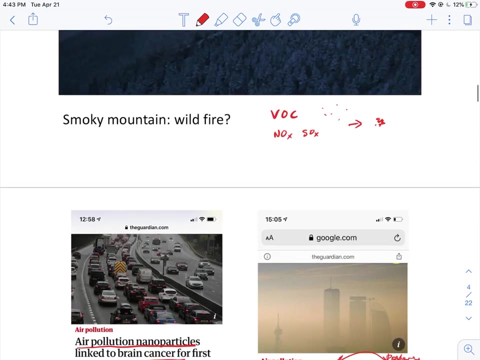 other effect, that's called the indirect effect, where the particles or the material matter can form cloud droplets and further form clouds to reflect the radiation. okay, so this is how the particular matter can influence the climate. so you can see that there is a reason why we regulate the 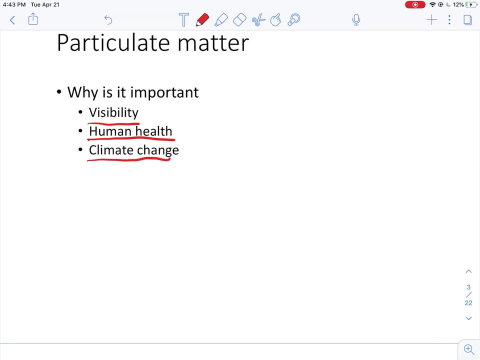 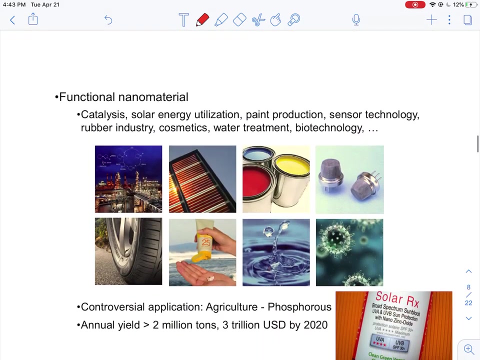 pm as a criteria or pollutant right. so it affects the visibility, affects the human health and also affects the visibility and affects the human health and also affects the visibility and affects the effects the climate change. so once we know the harmful effect of the pm, so there are also some. 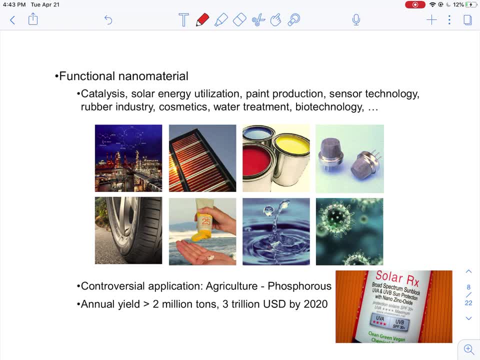 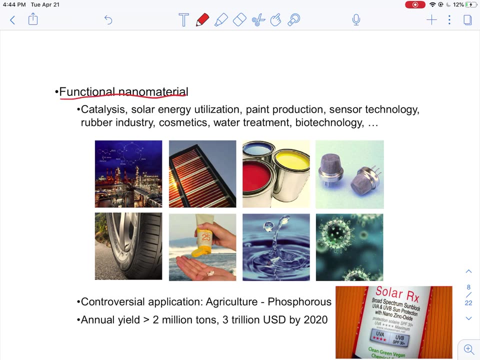 benefits of particulate matter. so here not only they're bad. so basically we know that pm may be bad, but actually they can also have some beneficial applications. for example, people have been using these functional nanoparticles for a long time, so we can use that for in industrial catalysis. 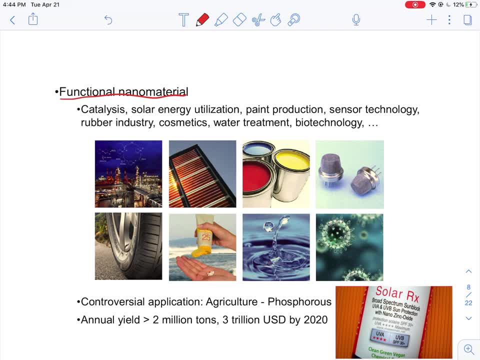 solar cell utilization, solar solar energy utilization. we can use them in paint. so next time when you buy paint and try to paint your house, you can have a check on the contents. there are nanoparticles inside. we can use particulate matter to make sensor right. we can add them into. 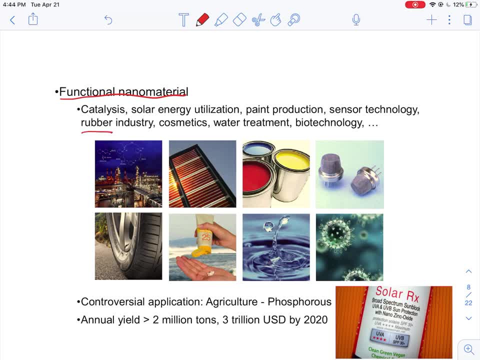 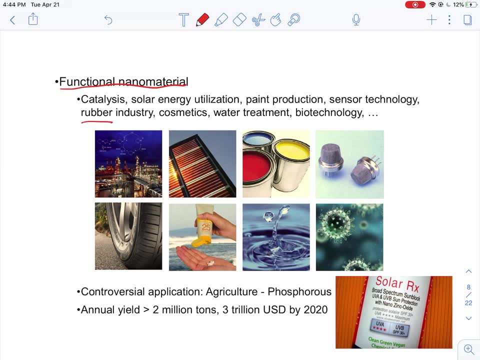 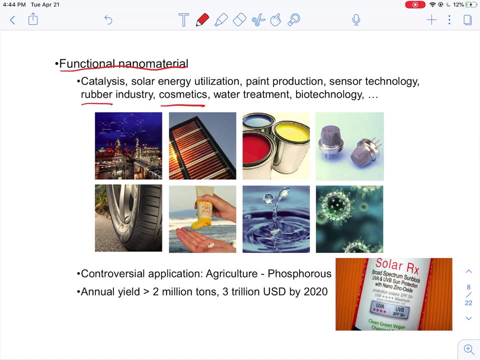 rubber to make the rubber more durable. right, because basically we put a lot of carbon black nanoparticles into the rubber to make the tires run for a longer time, and we also use them in cosmetics. right, so this is a picture of the sunscreen, but actually, if next time we buy the sunscreen, you can see that they will typically. 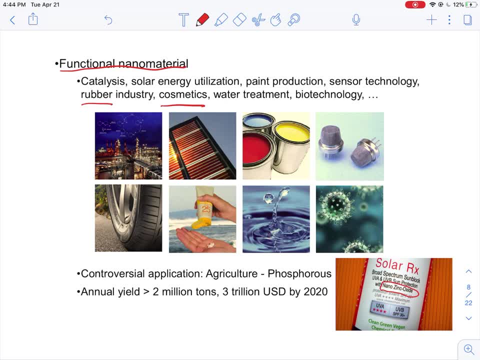 label that they will put in nano zinc oxide or nano titanium dioxide into the, into the sunscreen. this can enhance the reflection of the radiation from your skin right. we can also use them in water treatment, so we heard a lot on the wastewater and water treatment there, so we can use that for disinfection. 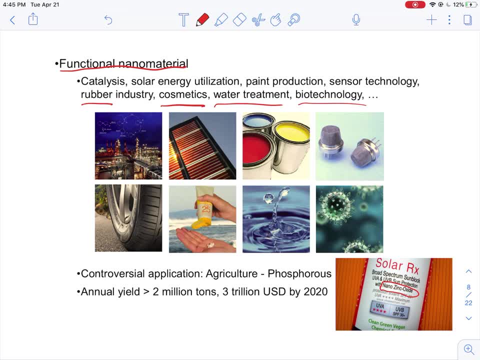 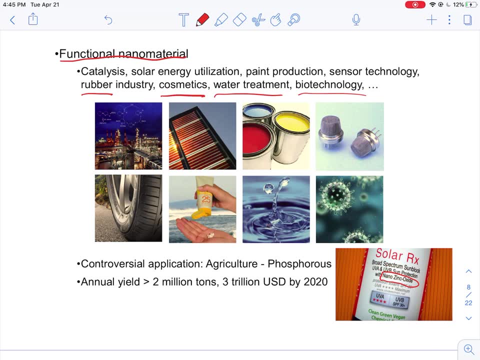 and then we can also use them in biotechnology and actually um. recently there are also some controversial applications. for example, we can use the nanoparticles as nano fertilizers in agriculture. we can boost up the yield of all these crops. but people may also feel concerned that they may get into our digestion digestion system right, further harm our body there. 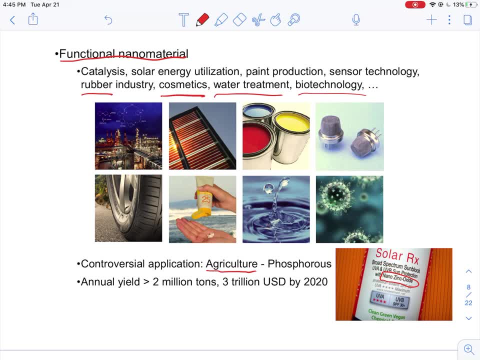 so, but that's still an open field. people are doing a lot of research on that, so people are predicting that by the year of 2020, the nanoparticle in the market can create a profit of around 3 trillion in the market there. so you can see that this is also a very 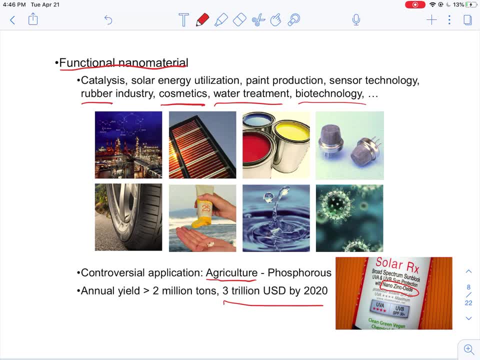 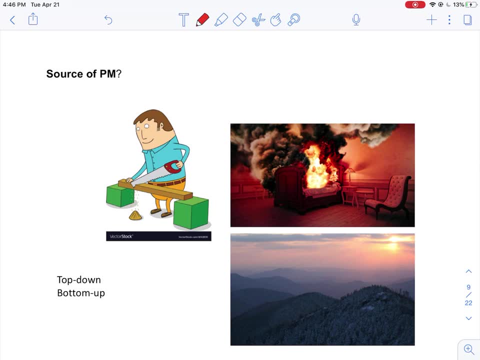 promising technology by using the particular matter from the industries. right. so we know about b3b5, Vega charging no α, α, α, ε ν and α δ army cell. there is a lista of smis ginger bee anxious ises, So there can also be a bottom-up approach, right. 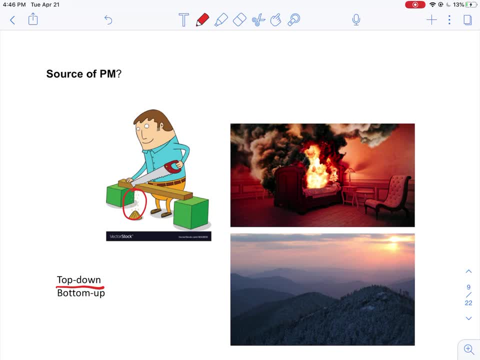 So, for example, we're lighting up a fire on our couch. You're seeing a lot of smoke here. So the smoke is not a part of the couch right? So by tearing the couch apart, we're not going to generate these smokes. 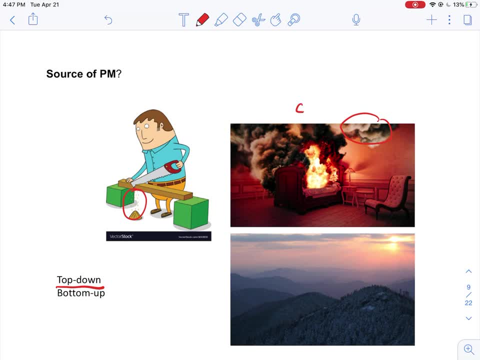 So the reason why we see this smoke is because of the carbon contents or the hydrocarbon content in the sofa, in the couch, get oxidized or get combusted right And they're not combusted completely. So because of that, we're forming a lot of particles containing carbon inside. 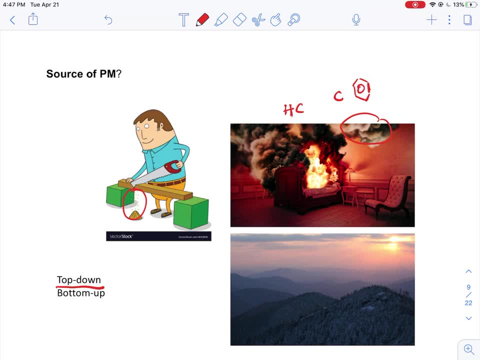 or the pH and the polyaromatic carbon right. So basically these will get mixed right, Form stable clusters of molecules and then form these particles. So this is a bioparticle. This is a bottom-up approach. So we also mentioned that the Smoky Mountain is also a bottom-up approach. 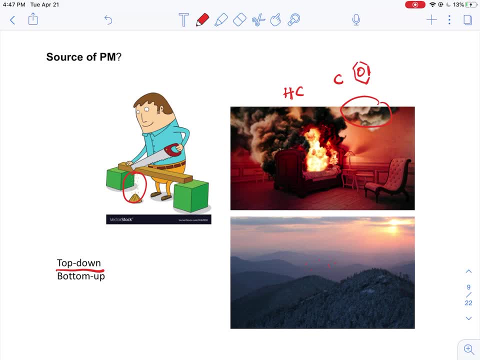 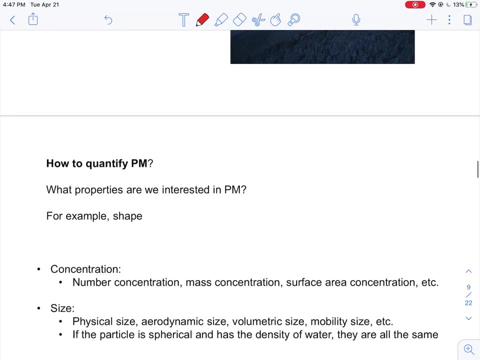 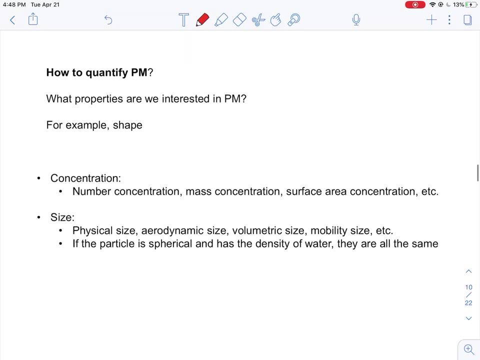 because originally there are just gas species And when they mix together they form stable clusters of molecules and then they can form particles, right? So basically, that's some background information on the particulate matter. So how do we quantify the particulate matter? 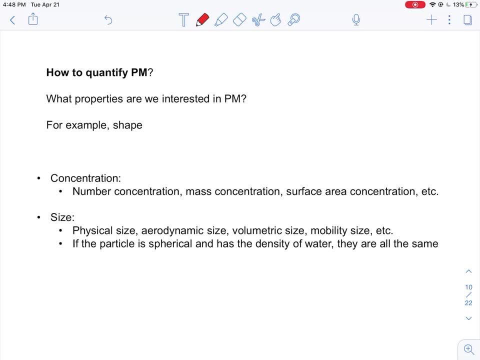 I mentioned that it is a very important air pollutant And we need to, of course, we need to be able to measure. measure them so that we can quantify or set up standards to limit their emission right. So what properties are we interested in? the particulate matter: 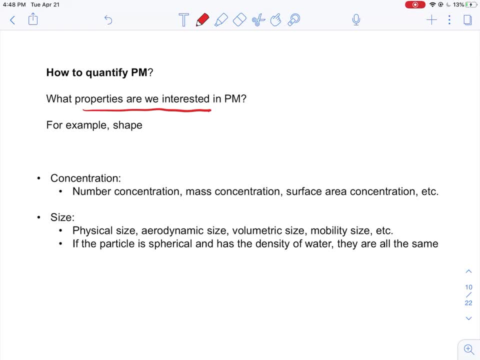 So, for example, we may be interested in its shape, because if they have a blade shape, then they can penetrate into our respiratory system and easily hurt our body right. So if they have a spherical shape, then it's less likely to directly harm our respiratory system. 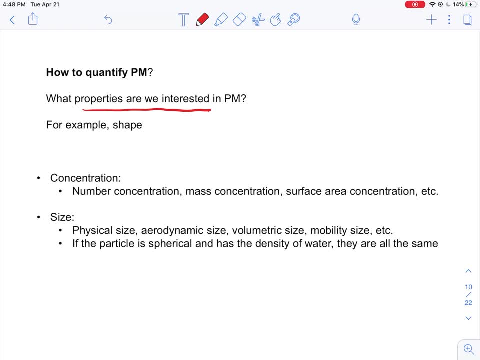 So actually the most important properties of the PM are its concentration and its size. So in terms of concentration, people will also measure, or there are different types of concentrations, right? People will measure the number of concentrations, so basically count: how many particles are there in the atmosphere, right? 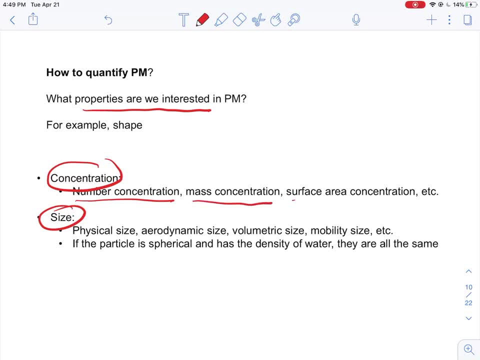 Mass concentrations. what is the weight of the particulate matter? Surface area concentration: right. So this is the a parameter that people are interested in: the health effect, because the larger the surface area of a particle, then the more active sites are there on the particle. 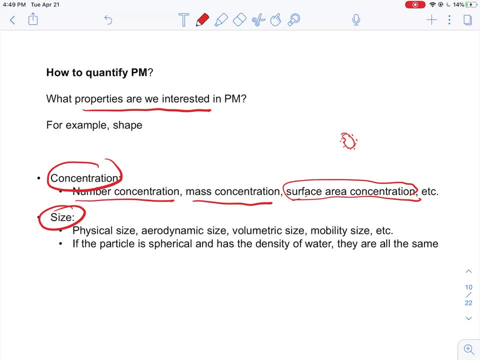 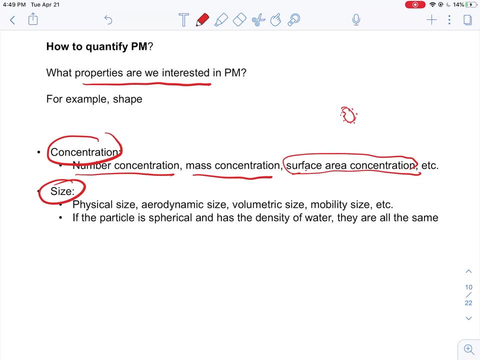 So there can be more. So basically that means once they get inhaled into the human body, then there's a larger contact area between the particle and the lungs, right. So people are also very interested in its size. So, in terms of size, 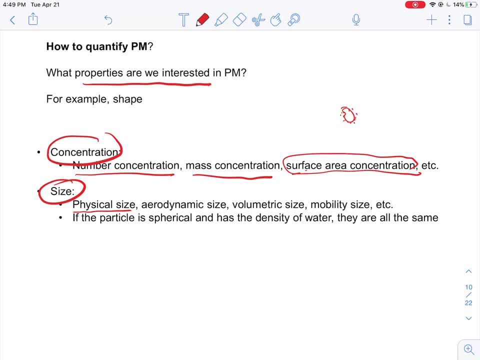 people have definitions of physical size, right. So what is the diameter? aerodynamic size, how fast it moves, volumetric size, mobility size and so on. So, but if the particle is spherical and has a density of water, then all of these will have the same size, okay. 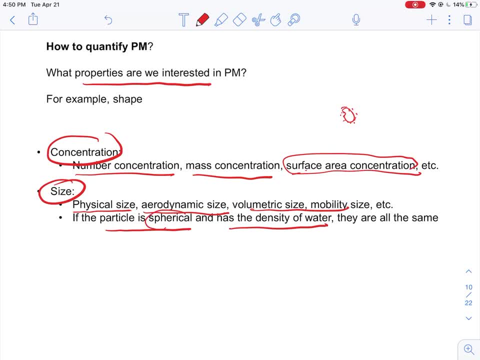 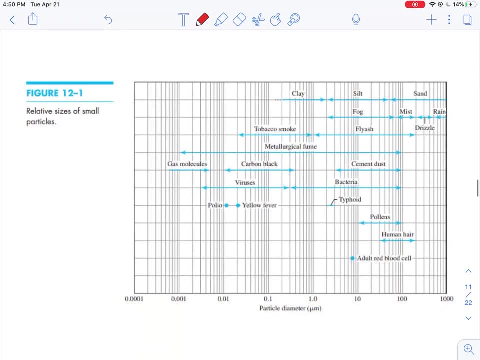 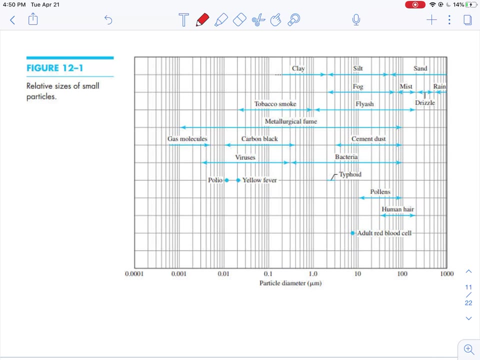 So in this class we'll just assume that all of the particles are spherical and have a density of water, So we won't consider other scenarios. So here there is a more or a detailed example of how particle size will affect its existing form. okay, 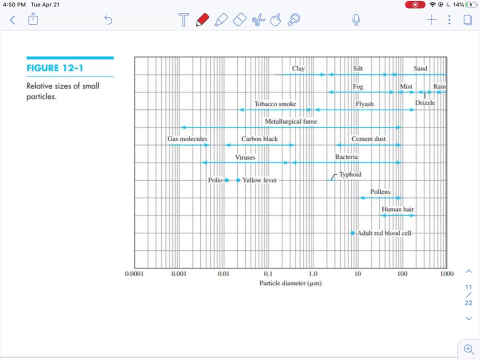 So here it's showing all different types of particulate matter and their corresponding particle size or particle diameter. So you can see that for viruses they have a very small diameter, right. They're in the range of what? 10 knot, maybe three nanometer. 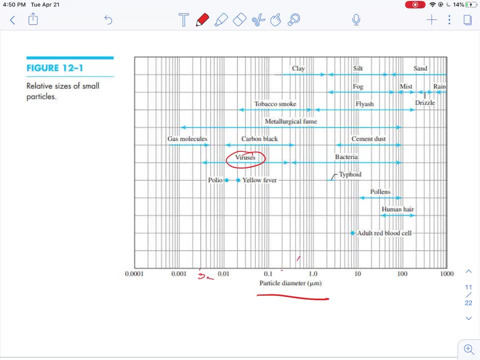 right, Three nanometer to, let's say, around 300 nanometer, right, And actually for the COVID-19 virus, it's around 120 nanometer somewhere here. okay, And then let's say we're talking about the fog. 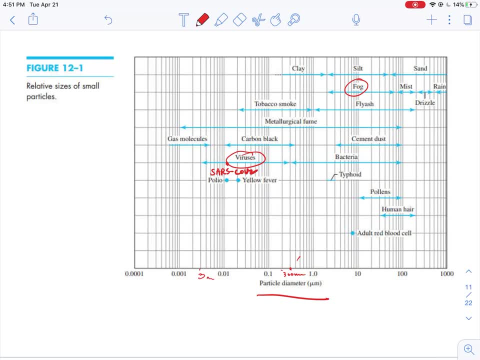 then the fog will have a very large particle diameter. It's around 10 micrometer. mist drizzle right. So different type of particles, they will have different sizes. Therefore, when we're trying to regulate the concentration of the particles, 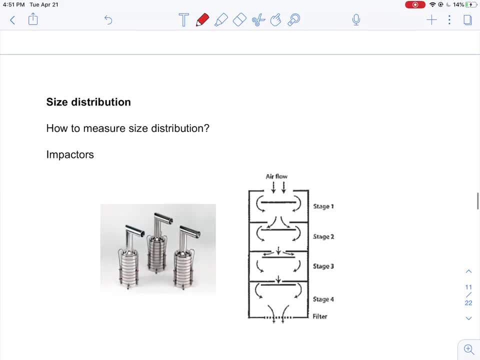 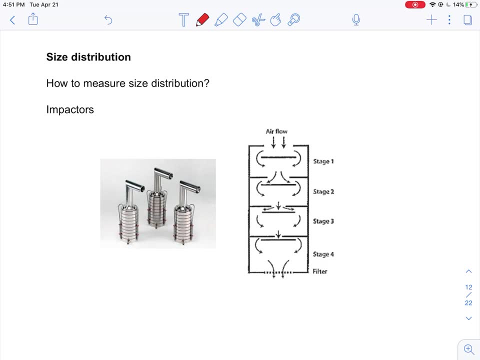 we need to know what is their size, right? So here I'm going to introduce a very simple device to measure both the particle concentration and the particle size. So we call this system as the impactor, okay, Or so people also combine different stages of this impactor together. 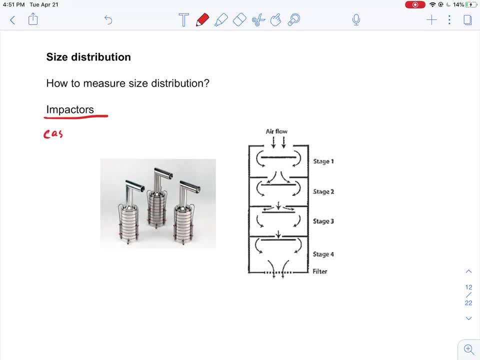 So we also call this the impactor. We call them as cascade impactors. So basically the cascade impactor or impactor uses the inertia of the particle. So let's say I just draw a single stage of the impactor. So the impactor is basically composed of a flow channel. 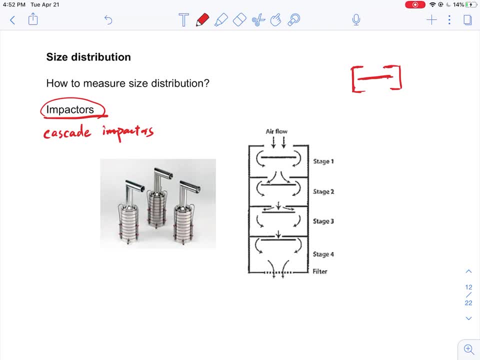 and then there's a stage in the middle. okay, So what happens is that we can introduce high-speed air flow going through the entrance of this impactor, And typically they will look like cylindrical shape. right, This is the inlet, okay. 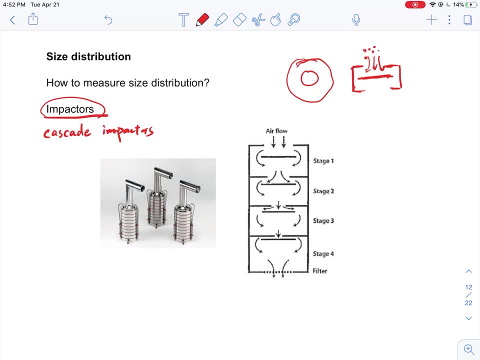 So while we introduce this sampling air or the ambient air inside, we know that there are particulates. So for the larger particles, because they have a larger inertia, they will just get impacted or get collected on the stage here, While for the smaller particles they will just follow the streamline. 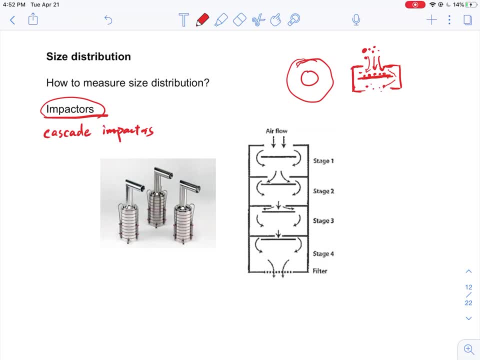 and then get escaped from this stage. right, We're going to have smaller particles, that's at the exit of this impactor. okay, So basically, we can create a second stage, let's say the stage two here. So you see, what I did is I can shorten this opening of the air, right? 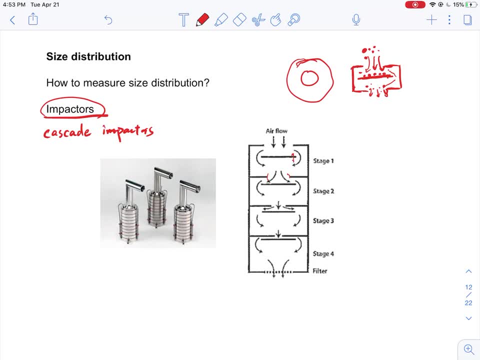 And at the same time I will lift up this stage, or collection stage, here to form this stage two. So what happens is that, let's say, after the first stage we're collecting these larger particles And then the escaped particles will have a smaller size. 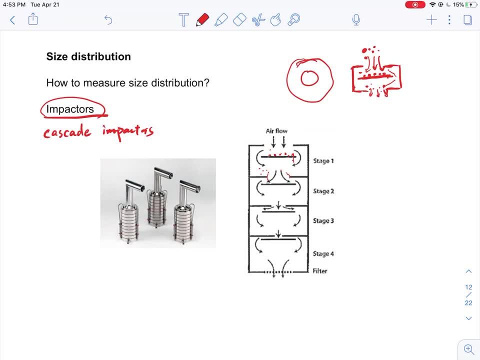 compared to these larger particles right And at the second stage, because the velocity of the particles becomes larger, so these smaller particles will pick up a higher inertia. So what happens is that among these particles, the larger ones will get collected here. 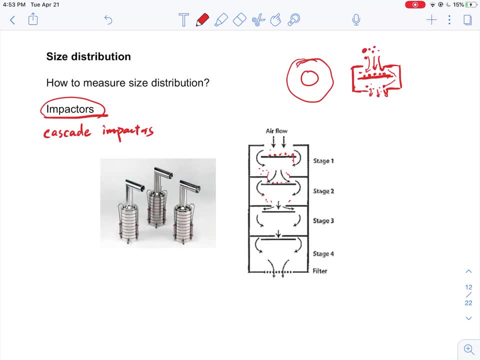 while the smaller ones will get escaped. So further we can have the stage three, stage four. So this is stage by stage. we're going to collect smaller and smaller particles, right? For example, we can buy these cascade impactors. 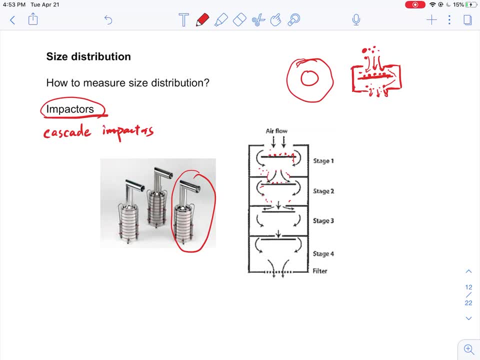 and each impactor will give you a size range. For example, the first stage will collect particles larger than 10 micrometers right. Second stage will collect particles from 8 to 10 micrometer right. Third stage, 6 to 8.. 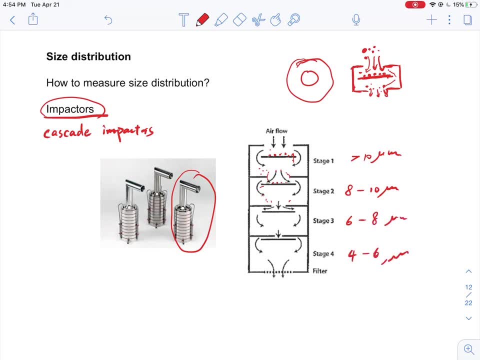 First stage, 4 to 6. So on and so forth. So by using this instrument and then after we collect, let's say the sample error for one hour and then we can disassemble that. So basically to pick up the stage here and then measure its weight. 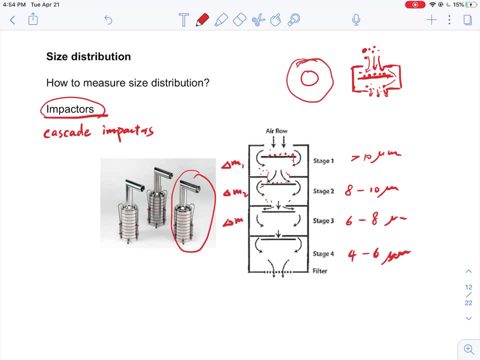 So we can measure the mass gain on different stages And then basically we know what is mass concentration in that size range. right, So we can easily plot a size distribution. Let's say, as a function of dp, what is the particle mass? 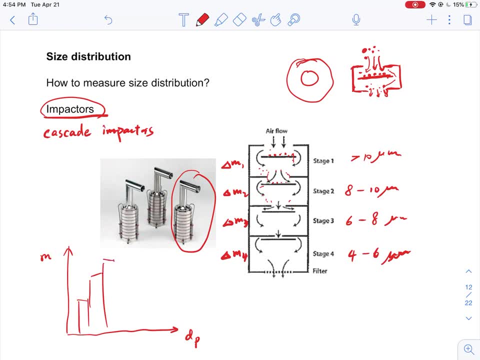 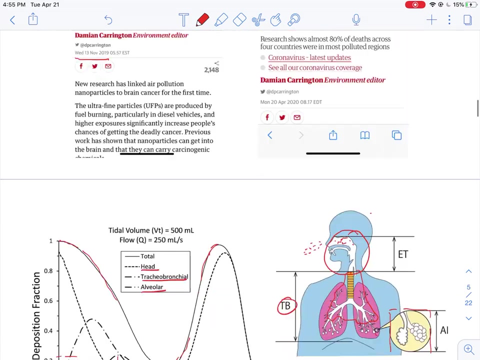 And they are going to give you a curve or give you a graph that looks like this: Okay, So this is how we call a size distribution of Pm. So the size distribution is very important because, as I have shown earlier, the size distribution will determine. 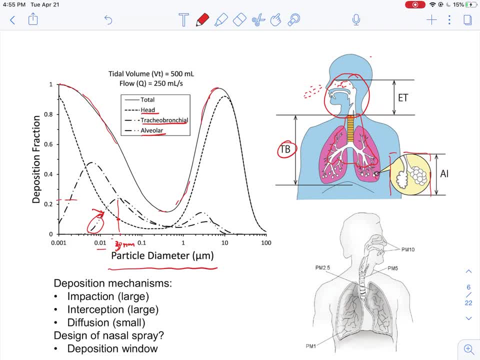 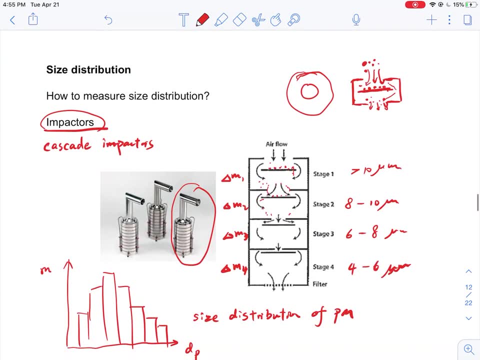 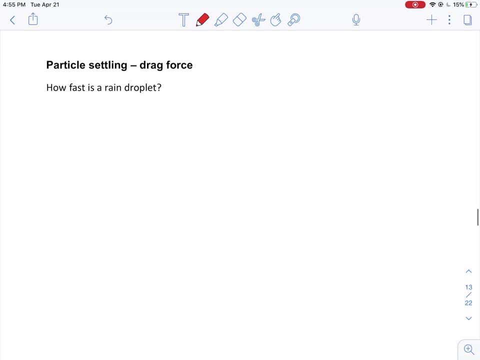 what is a fraction, or what is the amount of particles that's getting deposited in our lung, And it will also determine how efficient these particles are getting removed in the atmosphere or by different types of industrial devices. So when we introduce the particular matter, there's actually one important property of the particular matter that we have to talk about. 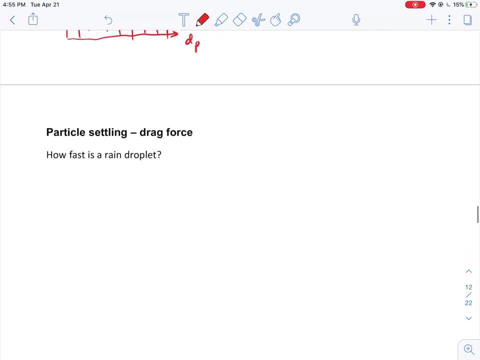 So in this class we're not going to go through too many equations, but this is the equation that I want all of you to go through. So, basically, if we think about a particular matter or a particle that's suspended in the air, 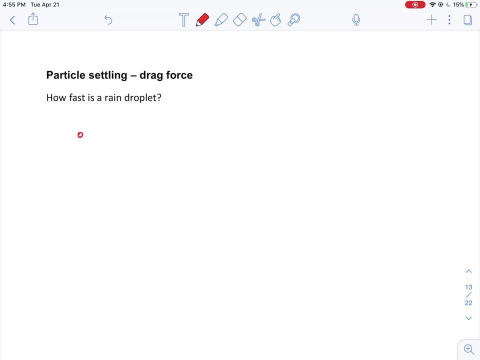 So, first, why is it going to suspend in the air? So why don't? for example, if we put a potato in the air, then there's no way that it can suspend, right, It's just going to fall down there. 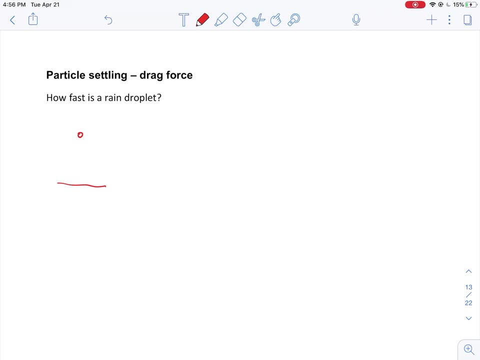 But why? the smaller particles can suspend there, right? So this has to do with extra force that's acting on the particle, And actually this extra force is drag force. So how do we know that the drag force exists? For example again: 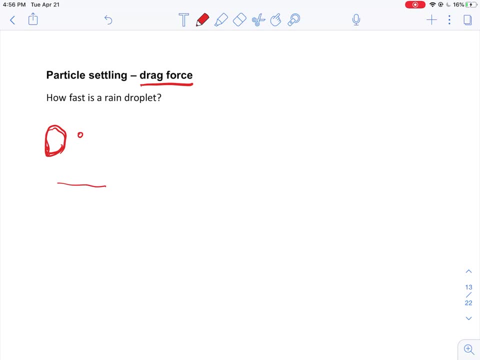 for the potato. we don't see a lot of drag force on the potato there right. So a simple example that I can give is the raindrops. So let's say, this is our ground right, And then we're seeing a cloud floating over. 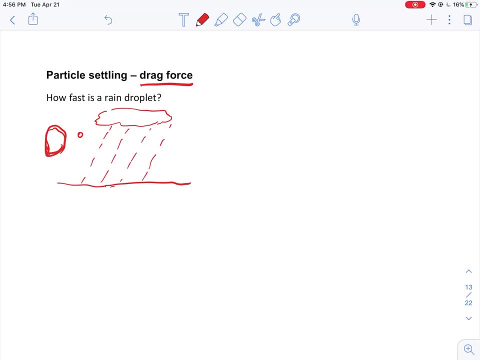 and then we're seeing rain here. Okay, So typically the cloud or the rain forming clouds, let's say we can assume that it has a height of around two kilometer. Okay So, two kilometer is a proper guess, but sometimes there can be further, higher or lower clouds there. 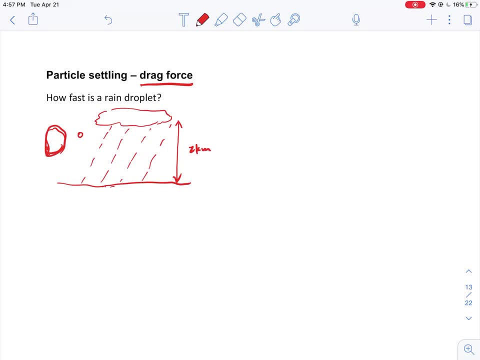 So let's assume that there's no drag force, right? So what that simply means is that let's say, if we have a droplet, that's probably around, let's say one centimeter, or let's say two millimeter. 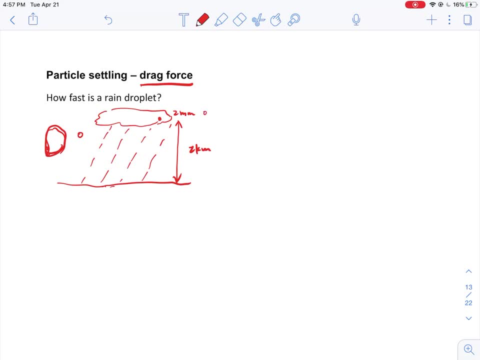 Okay, Two millimeter is a good guess of the rain droplet. So if we have a raindrop that has a diameter of two millimeter and then it's going to fall down, right, So if there's no drag force on it. 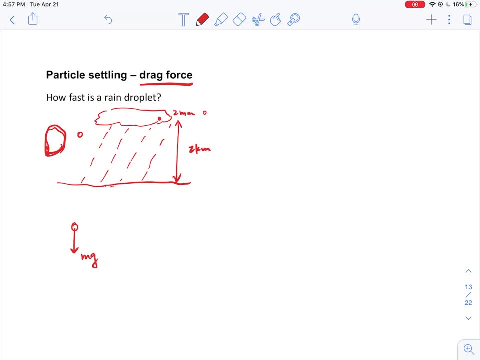 then the gravitational force is going to be the only force that's acting on the droplet right, So we can calculate what is the final velocity of this droplet when it falls onto the surface. So what we can do is we can set up the velocity equation for this movement of the rain droplet. 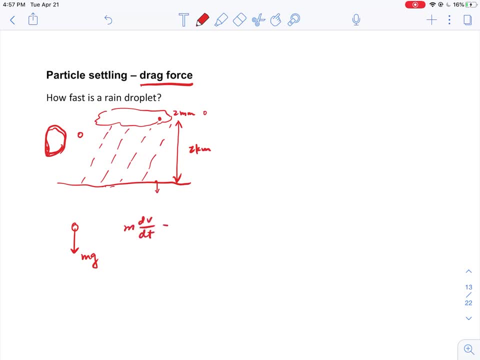 right. According to the Newton's second law, mdv dt should be equal to mg, where mg is the gravitational force or the gravity. Okay, So basically we can know that dv dt is going to be equal to g right. So further. 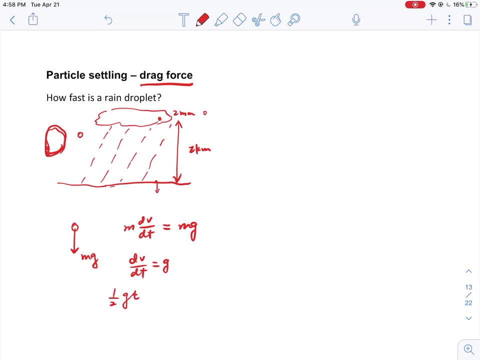 we can calculate that the distance that's traveled by this rain droplet, or the rain droplet is going to be equal to half of gt square. equal to height: right, The height is 2000 meters right And then further. we know that basically g. 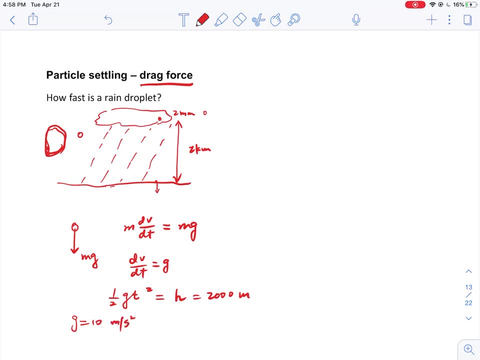 we can assume that it's just 10 meter per square, meter per second square, right? So we can find out that t square is actually equal to 400, right, We first get 4000 here and then divide by 10. That's 400,. 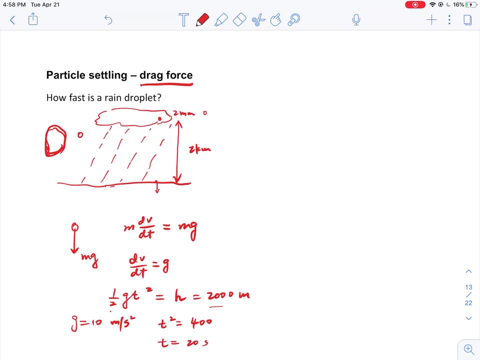 which means that time is around 20 seconds. Okay, So if there's no drag force, then it just needs 20 seconds for this rain droplet to fall down to the ground, To fall down to the surface. So what does that mean? 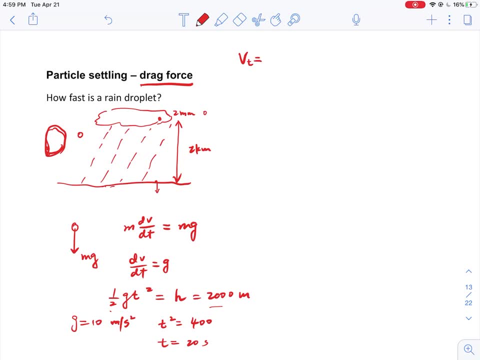 So it simply means that the final velocity of this rain droplet is going to be 20 multiplied by 10, which is basically g multiplied by t. right, That's going to be 200 meters per second. So is this realistic? So 200 meters per second is almost as fast as a bullet. 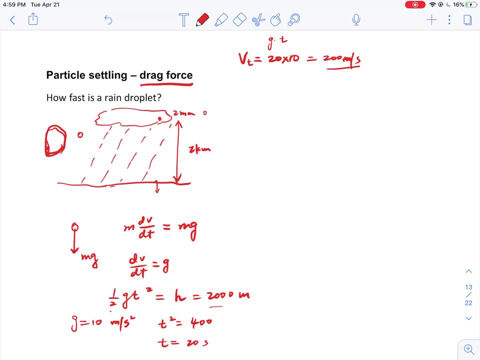 Okay, So if we go outside and then we never feel that it's bullet falling on us, right, We don't feel that pain. So actually, the, the raindrop: the velocity of a raindrop is typically around 10 meters per second. 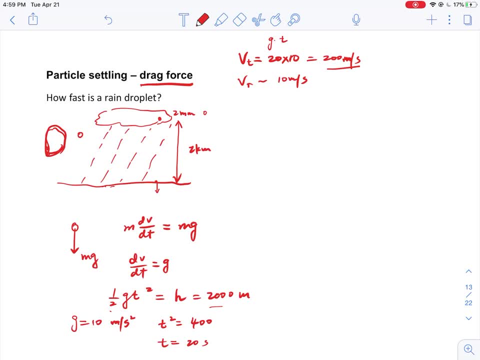 So what does that mean? It means that there have to be extra force that's acting onto this particle here. So this extra force is a drag force. So the detailed equations or the derivation of this drag force, I'll just skip that. So basically the drag force is equal to 3 pi mu dp. 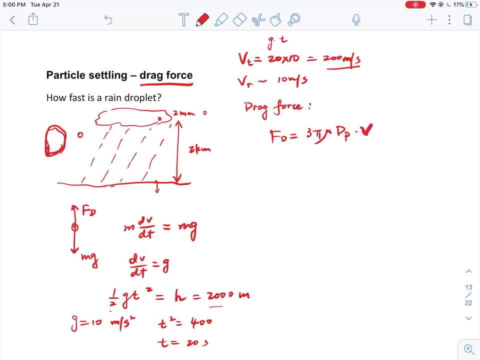 multiplied by the velocity of the particle. Okay, So mu, here is the, basically the air viscosity, right, The dp here is the particle size And the v here is the particle velocity. Okay, So basically, so, basically, this particle velocity is going to determine. 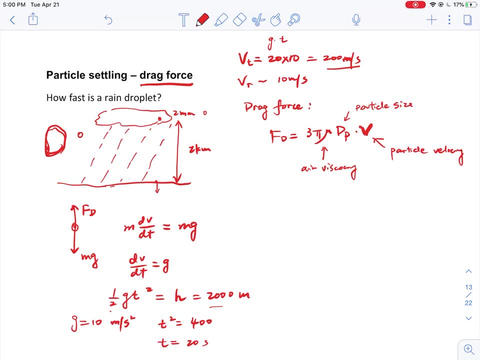 or determine how large the drag force is. So, for example, if you want to calculate what is the final velocity of this rain droplet, what we're going to do is we can set up the drag force equal to the gravity right, So we can get 3 pi mu dp. 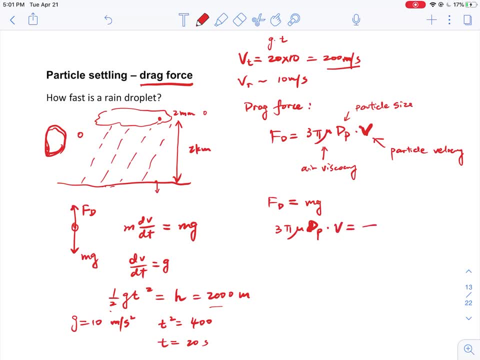 multiplied by v, equal to mg right, mg is the gravity And further. if we assume that the rain droplet is a sphere, we know that m is just the density multiplied by velocity, multiplied by the volume, right And further. 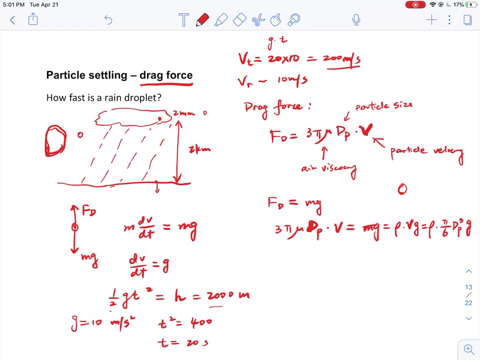 the volume is pi over 6 dp to the third g right. So we can cancel the dp cube right to form dp squared And then further we can calculate what is this final velocity there. So this final velocity here you can find out that it's actually dp squared. 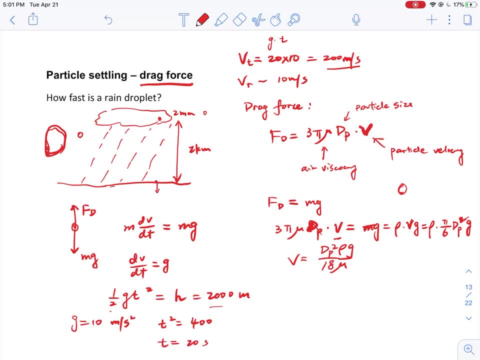 rho g divided by 18 mu. Okay, So you can see that the larger the particle size, the faster the terminal velocity, And also the larger the gravity and also the larger the density, the faster the terminal velocity for this rain drop. 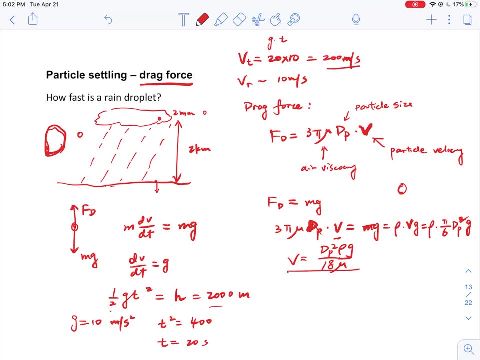 So now we have this equation, We can easily calculate how long it is for the particles to settle down, if we want to, if they are suspended in the air. So here I'll just give you a table to show what is the typical range for the particles. 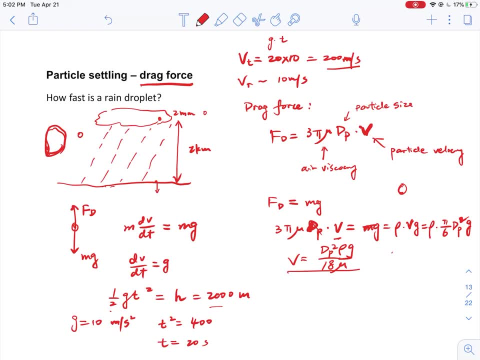 to settle down to the surface. Let's say that we're trying to settle down particles from 100 meters above the surface. Okay, 100 meters. Then let me give you a series of particle diameters, dp, and then we can calculate this v here. 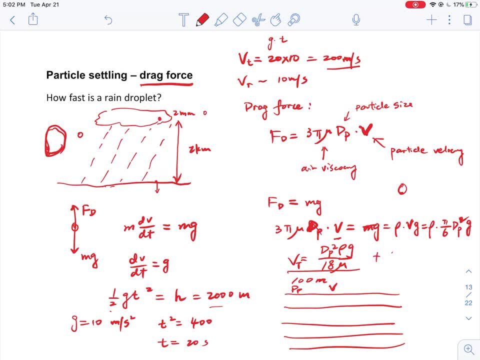 right. Typically we call this v as the vt, because this means it's terminal velocity, And then we can calculate what is the time it needs to settle down for 100 meters. So let's start from the smallest size, point 01- micrometer. 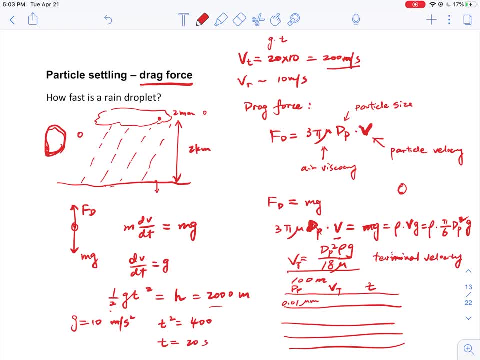 which is around 10 nanometers, So we can plug it in to calculate what is the terminal velocity. It's actually 6.7 multiplied by 10 to the minus 8 meters per second. that turns out to be 48 years. okay, for 0.1 micrometer it needs around 44 months. 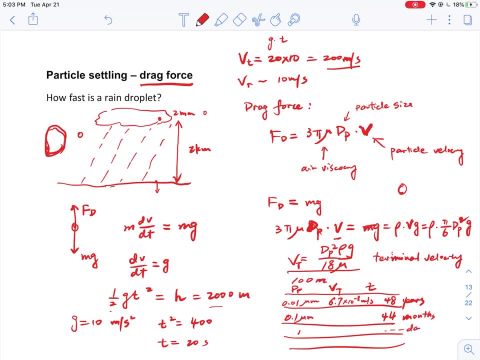 okay, one micrometer. you can calculate that later, but it needs days. okay, right. and finally, for a hundred micrometer, the particle size has to be around 5.2 minutes, right? so you can see that the larger particle size, the faster it can settle down. so now you. 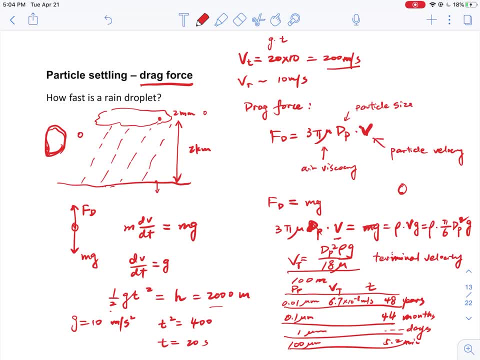 can know why the particulate matter can suspend in the air, right, it really depends on the size. if it has a really small size- right from 10 to 100 micro meter, 10 to 100 nanometer- they can suspend for very long time in the air. 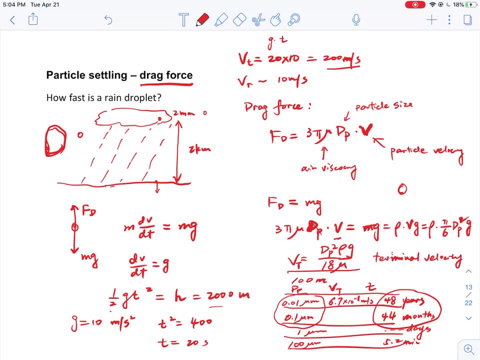 the air right. so now you can also start to relate that with the COVID-19. so people talk about how the aerosols can transmit the virus by speaking or singing, right by coughing. so if we generate small particles enough that can be in this range, then they can suspend in the air for a relatively long. 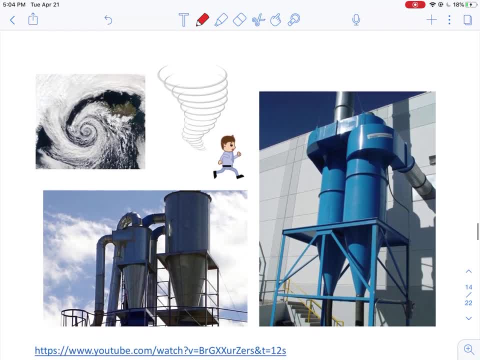 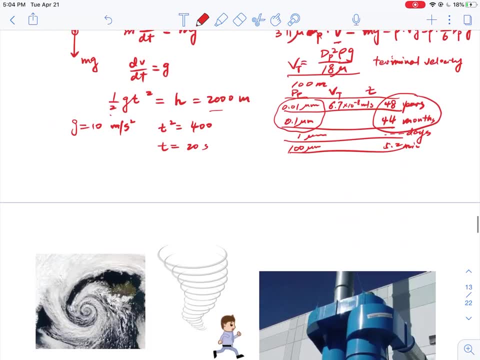 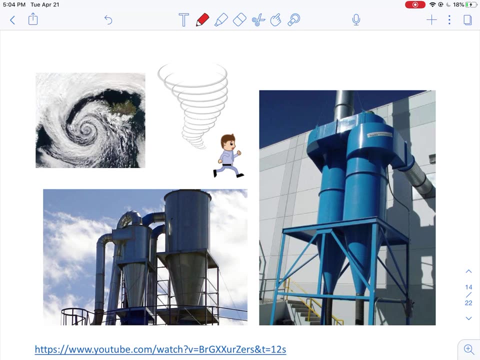 time. okay, so this is basically the backgrounds on the parameters related with the particular matter. right, so we can also introduce on how we can remove these particular matter from industrial processes. so the first one we should learn about is the cyclones. so basically, the cyclone is using the same concepts. 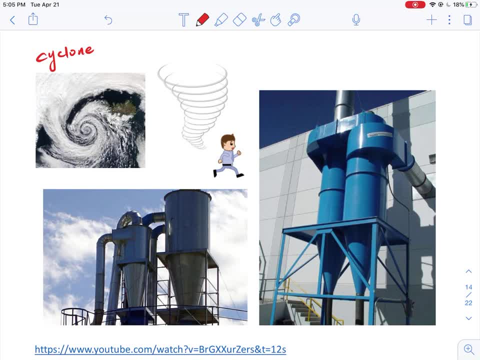 that which is the system. like Fi週, the nature, right. So whenever we see tornado coming on- at least we see them on TV- we can see that it's going to spin something out, right, Spin some objects out of it, simply because these 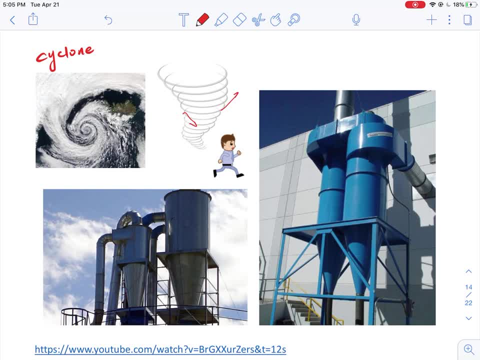 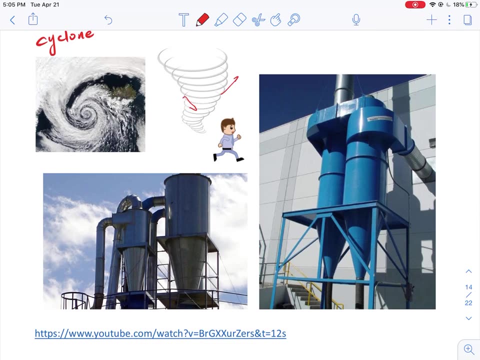 larger objects or the heavier objects, they don't have the centrifugal force to sustain this. rotational force here, rotational pattern here right, And we can basically use the same concept to remove particles. So what happens in a cyclone is that we're going to create this. 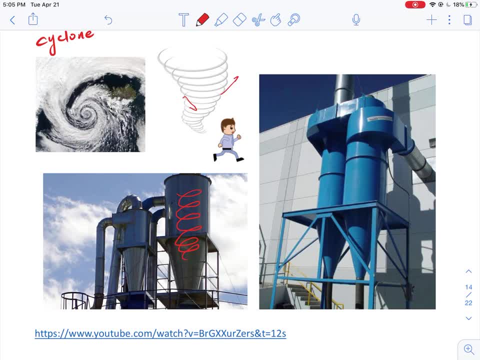 rotational movement in this device here, right So there's a lot of strong rotation, right So the larger particles will just get spinned out to the wall of the system And then at the end the cleaner gas stream will go through the center of the system and then go out of the system, right? So once the 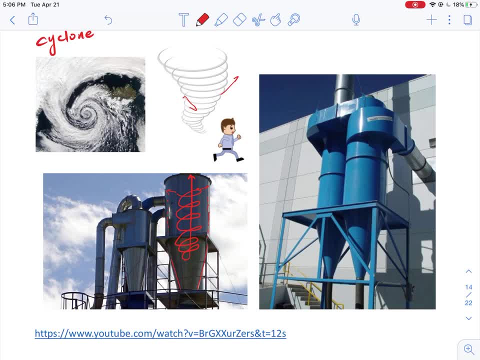 particles are getting spinned onto the wall. then they can further get collected by this cone shape here. So here I also have a short video on how the cyclone works, And if you're interested you can also click it and then take a look. It's. 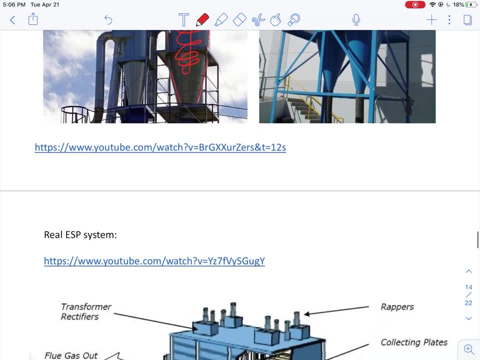 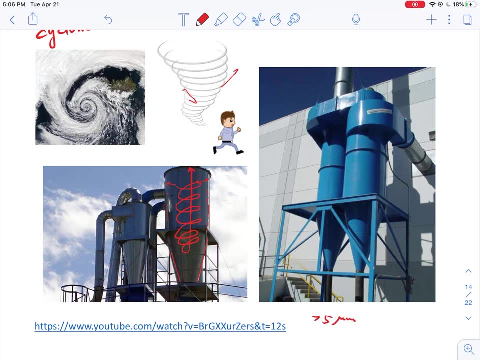 just a very short video. It's like one minute. okay, So typically the cyclone can remove particles larger than five micrometers. So you see that the cyclone basically uses the particle gravity or particle inertia. So the higher the inertia, the higher the inertia, So the higher the inertia. 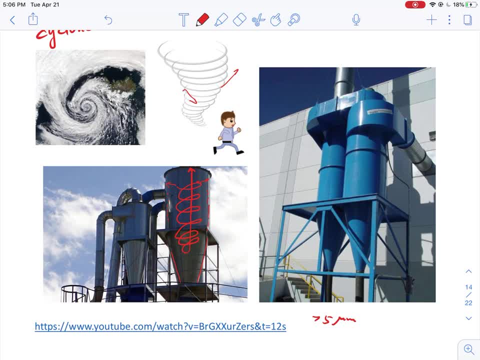 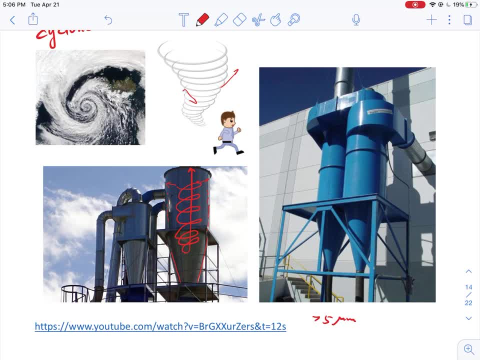 We know that smaller particles can suspend in the air for a longer time. We have to remove them before we emit it into the atmosphere. And, by the way, a lot of industrial processes emit a large quantity of particular matter, For example, the coal combustion: We're burning the coal and then 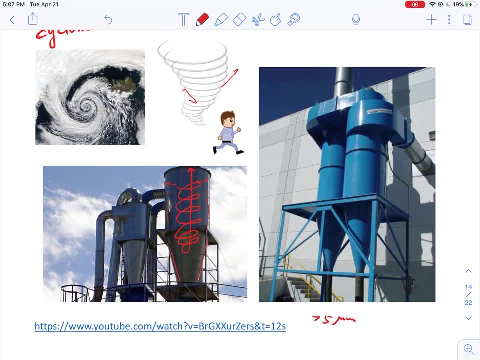 the carbon inside the coal may not get burned completely, Or there are metal in the coal, So basically those particles can get emitted in large quantities from the coal-fired power plant. So that's why we have to use these PM removal devices to purify the air before we emit it into the atmosphere. 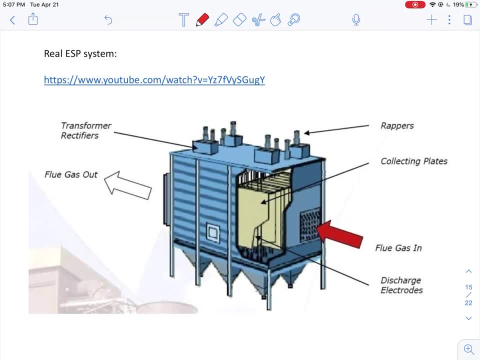 So for the smaller particles, what we're going to use is a system called the ESP. So basically the full name is the electrostatic precipitator, So electrostatic precipitator. So that's why it's called ESP. So what happens in an ESP is that we're adding one more mechanism to remove the particles. 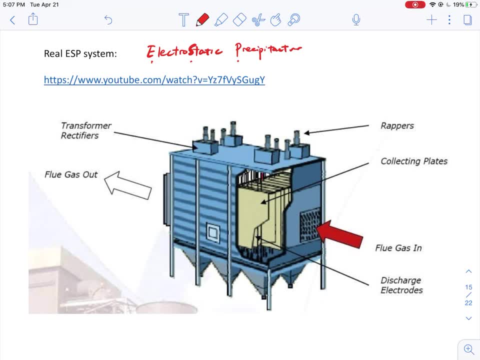 We're going to use electricity. So basically we have these very thin wires- ESP, We've got mechanical갔 that emit a lot of charges into the space, and then we have these plates that are carrying the negative or opp series polarity compared to. 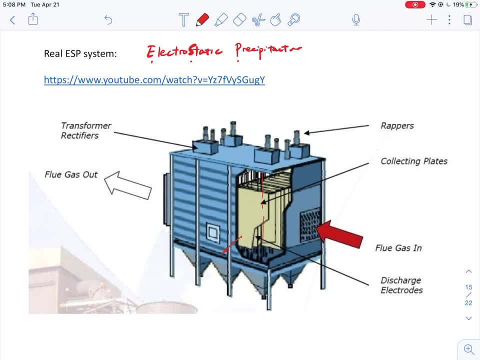 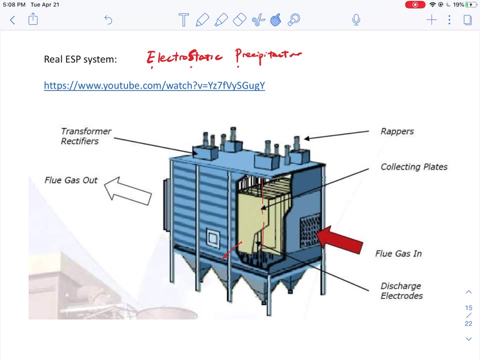 these wires. So basically we're creating a really strong electric field and then the particles can get charged and collected by these plates. So maybe we can go through this short. Eh E есте비. googlete short link very quickly, So it seems that it's not letting me to click it. 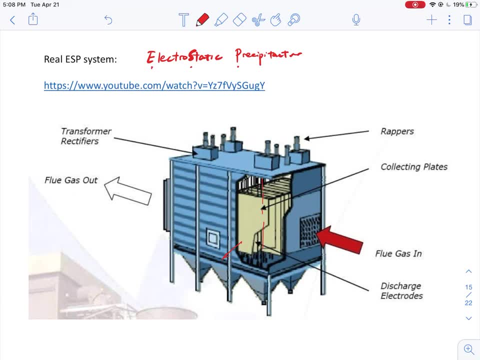 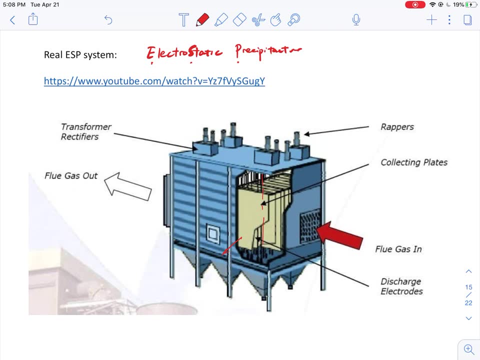 So maybe it will be better if you can go through these short videos after this class. So, basically, the ESP uses the electrostatic force to remove the particles in the flue gas and it has a very high efficiency to remove the smaller particles, For example, from 0.1 micrometer to 5 micrometers. 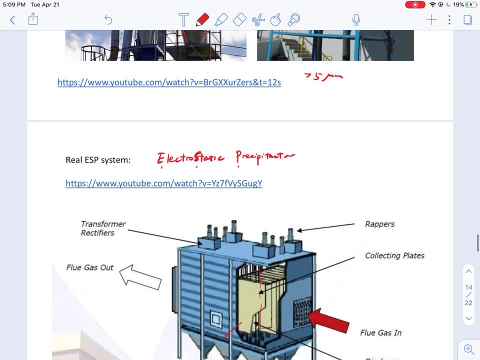 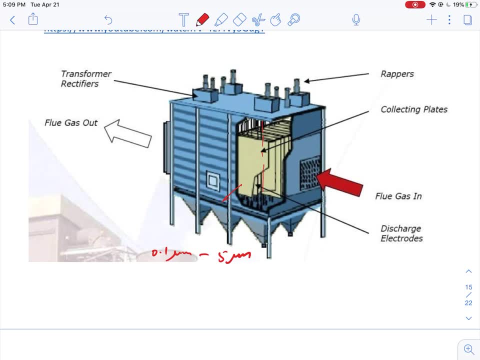 So that's why for coal-fired power plants people will combine these devices together to remove the particles. But for ESPs there is a special size range that it cannot really remove the particles with high efficiency. And even for these smaller size ranges they are not very efficient. 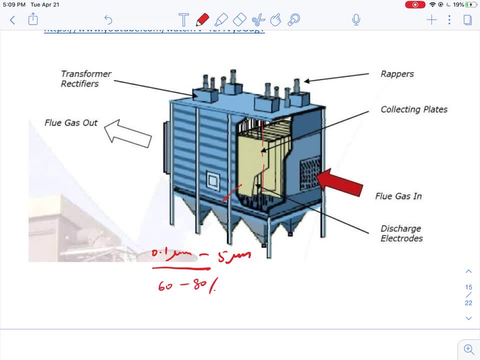 For example, the efficiency can be around 60 to 80 percent. So what if we want to create a coal-fired power plant? Or what if we want to create a particle removal system that doesn't emit any particles? So there's a requirement for these systems, because we're not only talking about the 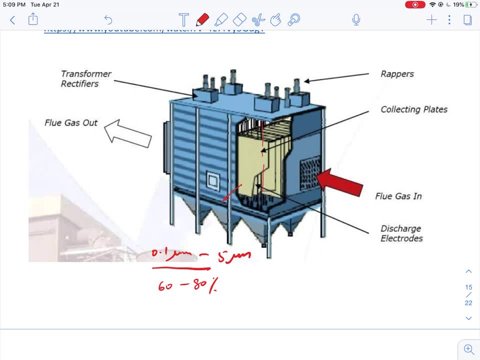 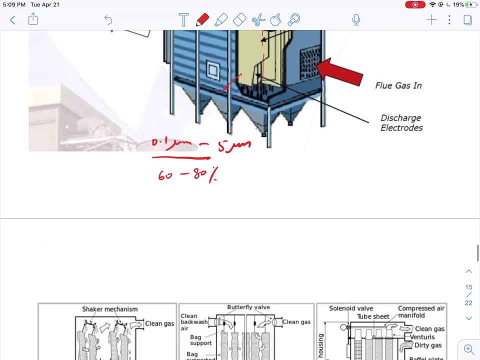 coal-fired power plants. So there are some industries that will emit toxic particles, right? So we don't want any of those particles, or PM, to get emitted into the atmosphere, So we want a high collection efficiency or removal efficiency for these particles. So that is the scenario when we have to use the filters, okay, 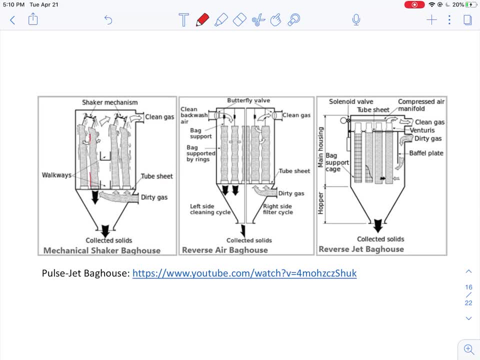 So there are different types of the filters. So basically, people create these bag houses So they just look like a bag right, And then they use the filter material to construct this bag And then, when the air goes through, the only way it can go out is from 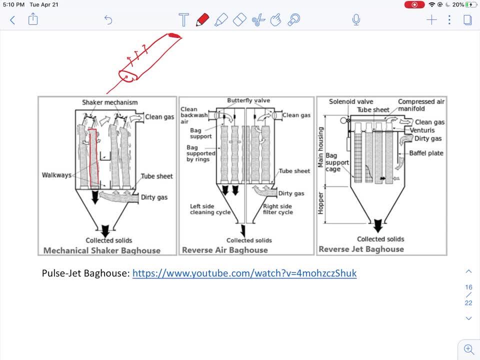 through the fabrics. So there isn't an outlet here. So the other end is just sewed there, right? So the only outlet is going from the sides. So now you can see if we introduce a dirty gas through these bag houses, right or the 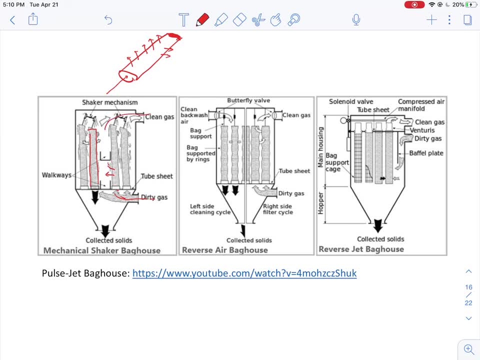 filter bags, then the clean air will come out from the side and then further get emitted from the device, right? So, yeah, it seems that the link here is not working. Okay, So it will be good that you can go through these short videos during the class, because 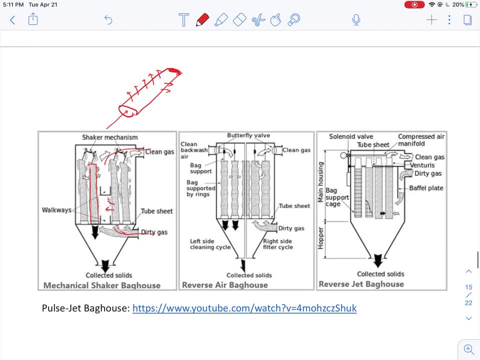 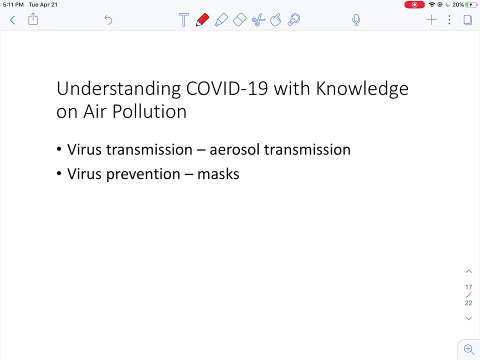 these are just like 30-second videos. You can get a better understanding of how the particle removal devices work. okay, So now, before we finish this class, I want to briefly talk about how we can use our knowledge on air quality or air pollution to look at this COVID-19 situation. 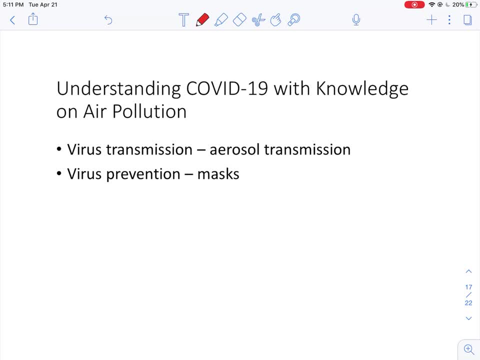 Because there have been a lot of discussion, right, So there are also studies showing that the mortality might be related with air pollution, So we're not going to see these. the effect of this air pollution on COVID-19 directly from these cases. 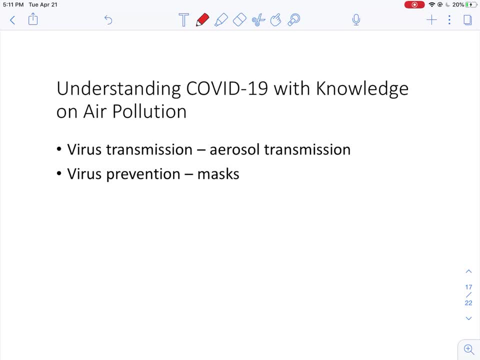 We're not going to see that from that aspect, But we're trying to understand the basically the transmission and prevention with our knowledge on air pollution. okay, So basically we can try to understand why, basically how the virus are getting transmitted in the air. 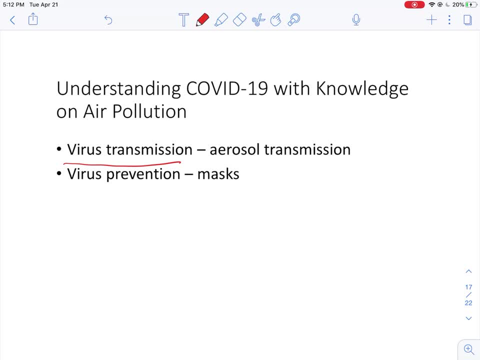 Because, basically, these virus are aerosols. right, Once we cough it out. right, they can suspend in the air. right So they can affect the transmission of these virus. right. So we can also talk about the virus prevention, where the masks or the, the filters, right. 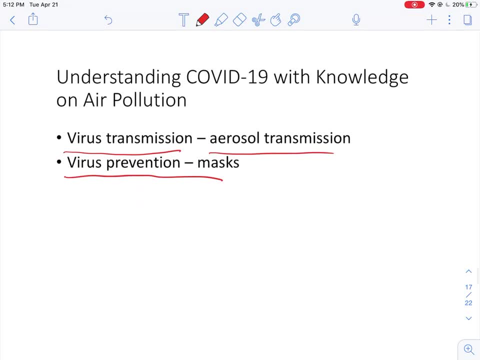 The filters come into the picture. So I'm just going to talk about the, the COVID-19, from these two aspects on how we can understand these processes with our knowledge on air pollution, And if you attended that panel discussion that I introduced or I talked about last week, 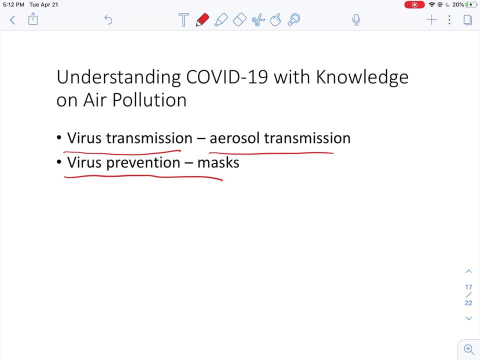 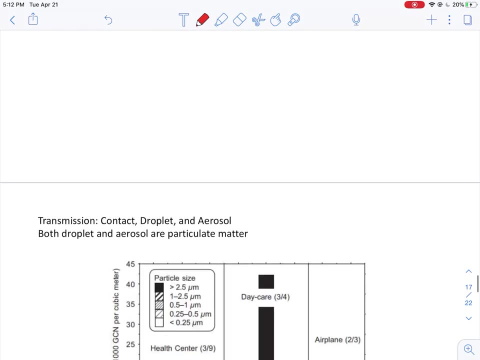 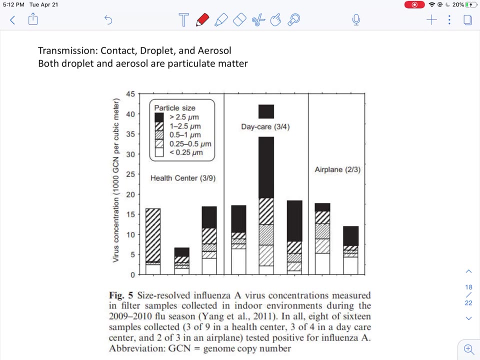 you can actually get more detailed information, And I hope that you got more detailed information from that discussion. Actually, I find it very helpful. So let's first talk about the virus transmission. So currently in the hospitals there are three ways of virus transmission or disease transmission. 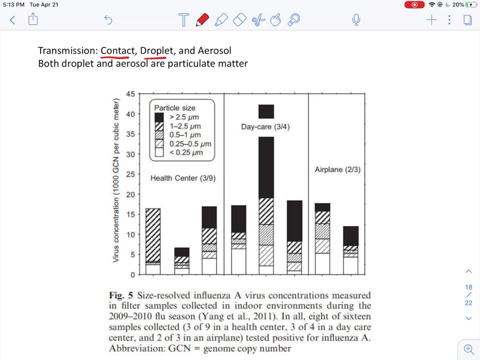 So there is a transmission mode called the contact transmission. There can be droplet transmission and aerosol transmission. So contact transmission basically means that you touch the patient or you touch the surface where the patient might have touched right, So that can cause the transmission of the virus or bacteria. 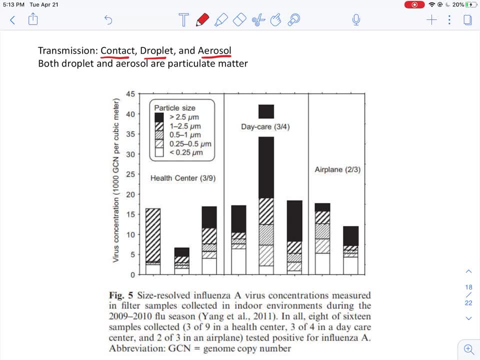 And then the person can can get infected. Okay, Okay, Okay, Okay, Right. So that can cause the transmission of these two things, right? So the contact transmission is the one that causes the virus or bacteria to get transmitted. So the droplet transmission means that you inhale the, the particles generated by coughing. 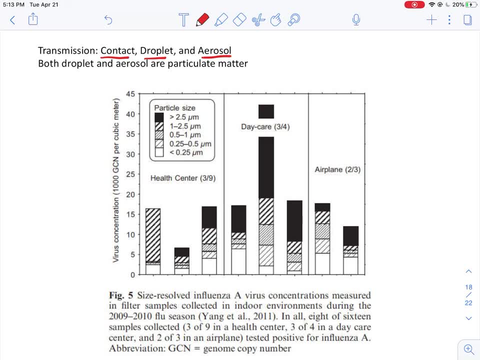 or sneeze, right. So typically these droplets are larger, right. It can have a size of a raindrop, let's say. or it can have a size of a fog, A fog particle, right. And then in terms of the aerosols, they're smaller sizes, right? 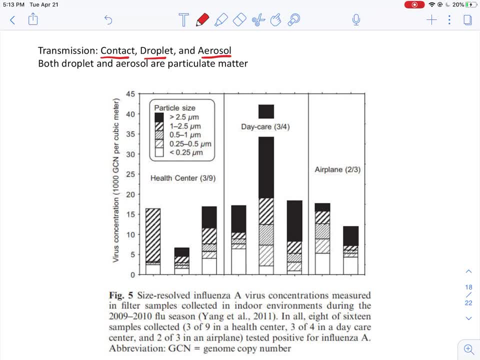 speak or people sing right. So in Washington state actually there's a case saying that people who attended a choir right got transmitted by attending that event. So you can clearly see that this COVID-19 may have some features of this process or this mode, so-called the aerosol. 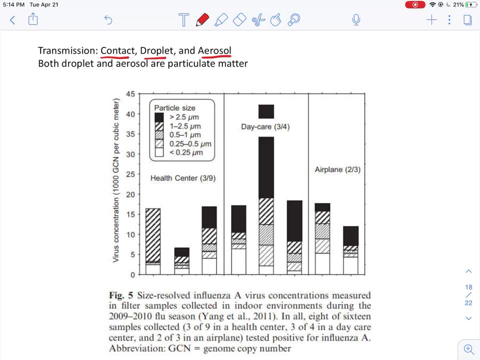 transmission. But from this class we actually find that there's no difference between droplet and aerosol right? So both of them are particularly matter. So that's why, in the aerosol field or in the air pollution field, there isn't a difference between the so-called droplet transmission or 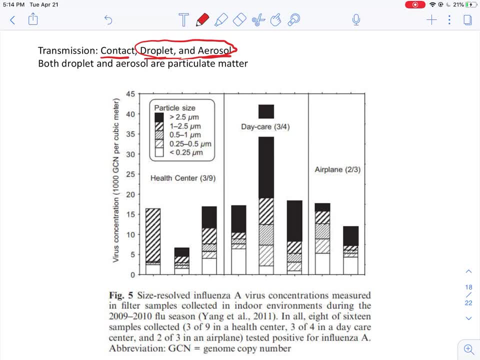 aerosol transmission. People may say that there's a higher probability that these particles or these virus may be carried by larger particles, Or they have a higher probability that they can be carried by smaller particles, But there's actually no direct distinction between the droplet or aerosols. So actually this classification is. 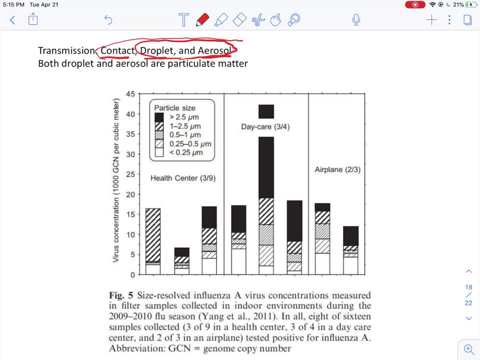 created from maybe tens of years ago or the early times of last century, because people haven't been dealing with these large pandemics for a long time. So actually it is quite expected to see that the whole research field might be reassessing this transmission. 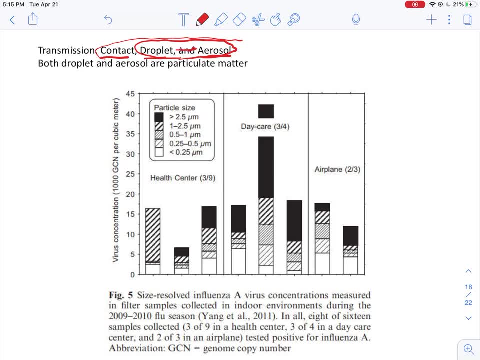 methods from a new angle, And even they might be combining this droplet transmission and aerosol transmission into one type of transmission. Maybe that can be called particularly matter transmission, Who knows? Okay, So we know that from this class both droplet and aerosols are particularly matter. 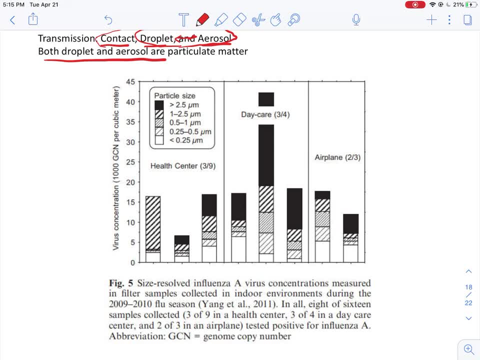 right. So here it's actually a little bit more complicated, but it's a little bit more complicated. So we know that from this class, both droplet and aerosols are particularly matter, right? So here it's actually showing a research study finding how aerosols, or how small particles, are important in terms of 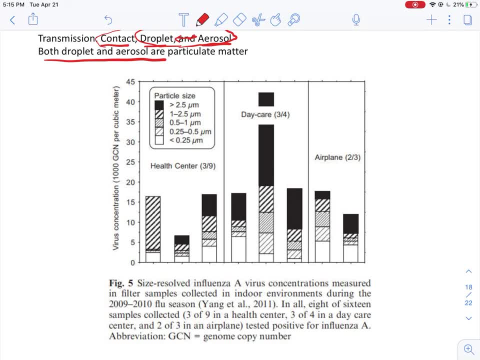 transmitting the aerosols. So this is a study that's conducted in different indoor spaces, For example, a health center, in a daycare and in an airplane right. So people basically use the impactor- cascade impactor- that I introduced earlier. right, You can collect particles with. 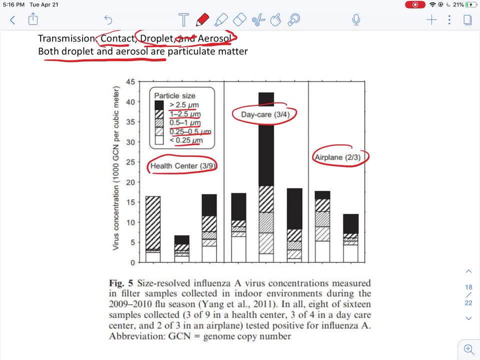 different sizes and then send those filter or send those particles to different places, And then these particles are collected, particularly into biological devices, So they can measure how many DNAs or how many RNAs are there in the collected particles. So what? 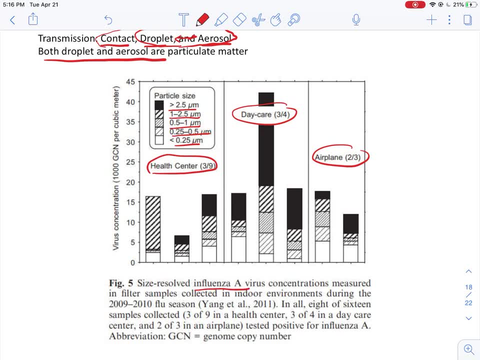 they find out is that they're testing the influenza A DNA or RNA. So what they find out is that actually, particles with smaller sizes, right below 2.5 micrometer they have a higher probability collected particulate into biological devices. so they can measure how many DNAs or how many RNAs are. 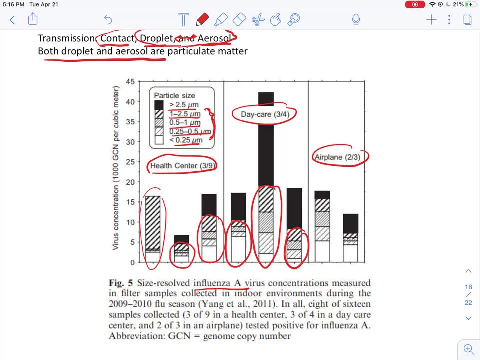 influenza A virus. okay, So only the black bars here represents the particles with sizes larger than 2.5 micrometer which can be in the range of the droplets. okay, So you can clearly see that the smaller particles are harmful. So aerosol transmission is important for the influenza A. 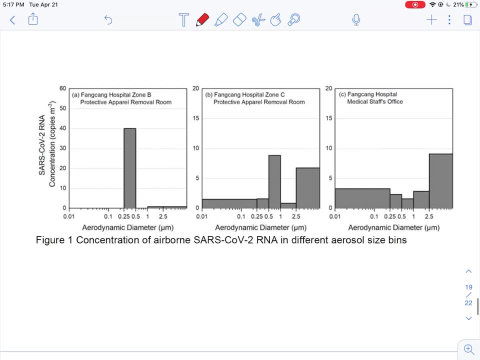 virus right. And specifically for the COVID-19,, people measure the SARS-CoV-2 RNA right. So we know that this virus is composed of RNA in its genes. okay, So this is what they did for the. again, for the aerosol sampling with the cascade impactor. You see, they measure the particles in. 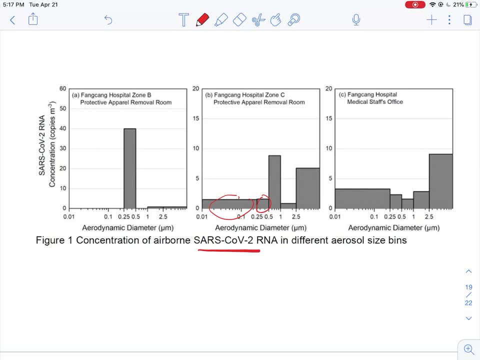 different size ranges. This is how we can directly relate with what we know from this class to do the sampling, right. So after they collected these particles and sent them to machines to measure how many RNAs are there, And you can see that they measure those RNAs in the range between 0.25 micron to 0.5 micron. right, This is the range. 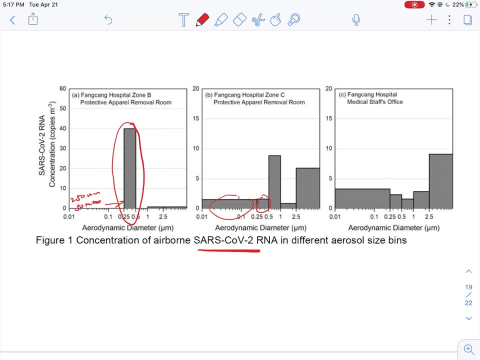 It's just 250 nanometer to 500 nanometer. So if you recall what is the size of a SARS-CoV-2 virus, It's around 120 nanometer, right? So the particles that's carrying this virus is not very large. 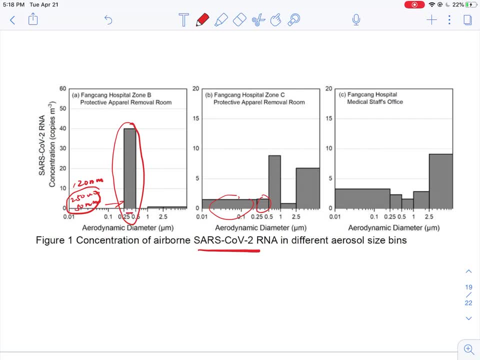 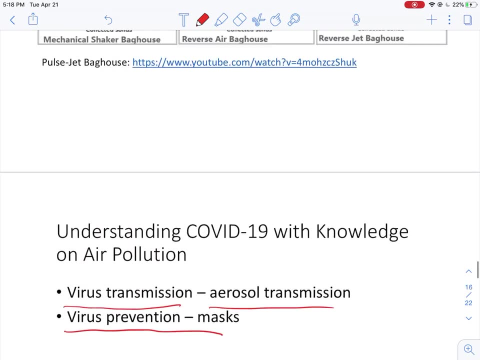 right. And if you further think, think back on what is the time that's needed for the particle to settle down. They can stay in the air for a pretty long time, right? So if you go back for 100 nanometer particle, 0.1 micrometer particle. 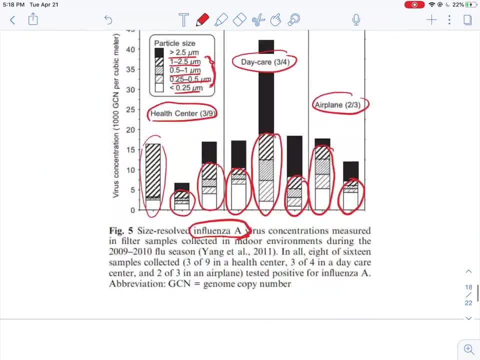 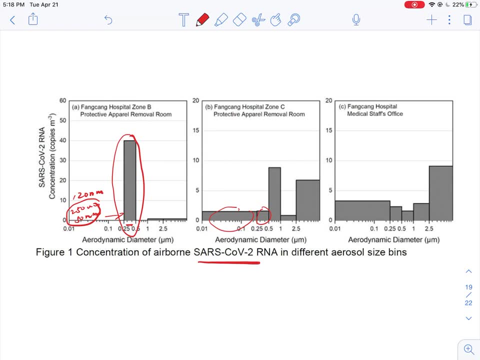 they can stay in the air for 44 months, right? I'm not saying that the SARS-CoV-2 can stay in the air for that long. Of course, the particles can stay in the air for a very long time, but 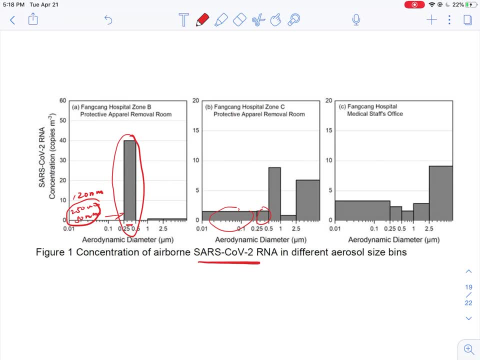 the virus also have a lifetime right. There is a viability of the of the virus, But more of more recent studies actually showing that the virus can stay in the air for a pretty long time. So there's a recent study showing that the virus can stay alive. 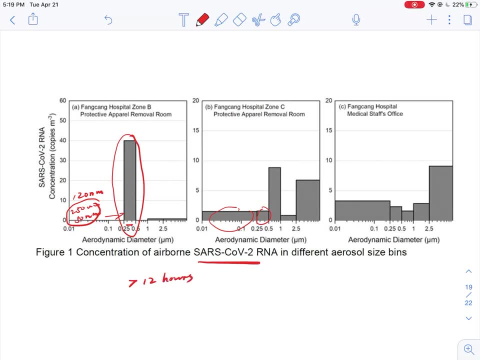 for longer than 12 hours- okay, For longer time. they haven't tested yet, but at least they can stay in the air alive for 12 hours, right? So you can think that this is actually a quite severe issue. So if we're staying in a room with a lot of patients carrying this virus, 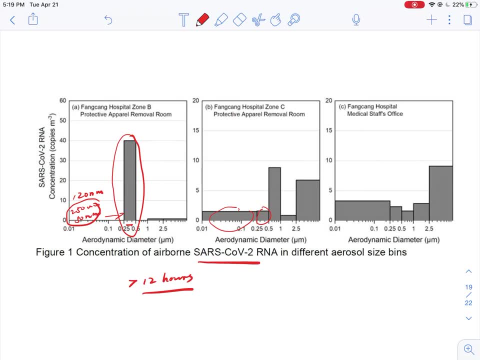 and they're all talking, speaking, singing right. If we inhale these particles, it's very likely that we can get transmitted, And it's not only showing that the virus can exist in the air. So actually they measure the virus in quite many rooms. 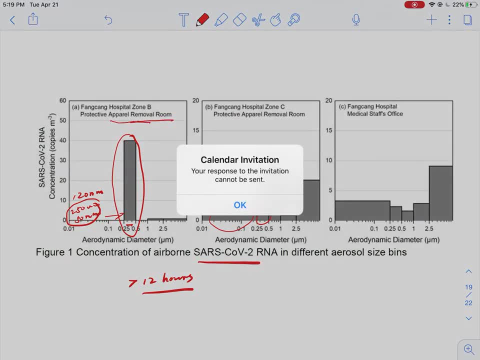 right. This is a hospital right. In the apparel removal room right There's also a protective apparel removal room and medical staff's office. You can, you can see that the measures, these, a lot of these samples, are actually in the smaller size range, And this is also. 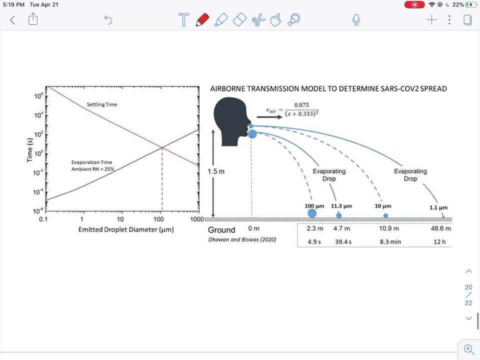 very concerning, okay. So if we look, look at a more realistic issue, right? So if people is sneezing, coughing, right, Generate a lot of particles. So one thing we need to know is that we we don't cough these virus in its pure form. right, Let's say this is a virus, right, It has. 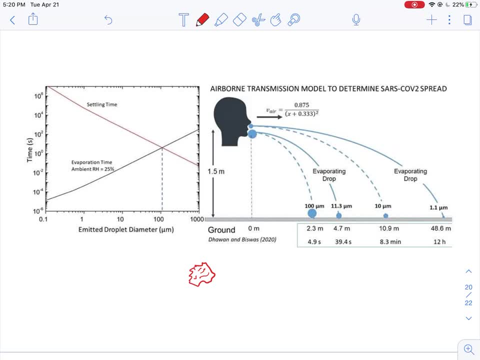 RNA strains inside. So we don't cough this virus in its pure form. right, Let's say this is a virus. right, When we cough, we don't directly emit these virus, because we know that there's always saliva right In our mouth. Actually, it's a cluster of droplets that's surrounding 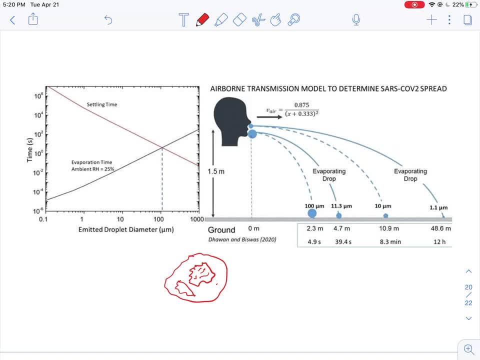 these virus. Now there can be multiple virus inside, right, So there's also protein, right. There can also be some salt right At the ionic species inside, So once they get into the air they can evaporate and then the water can get removed. 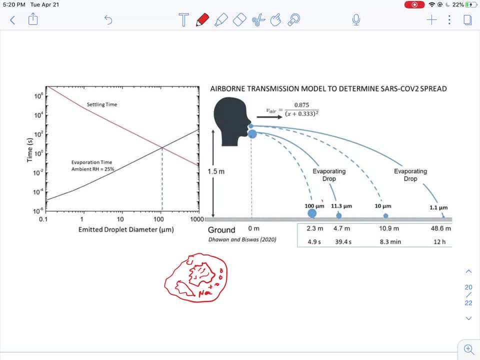 That's more concerning because, let's say, if we're coughing, we can emit um initially, for example, generate a hundred micrometer particle right. While they're being emitted out, they can also evaporate, So the water can can get out right, The particle can shrink. 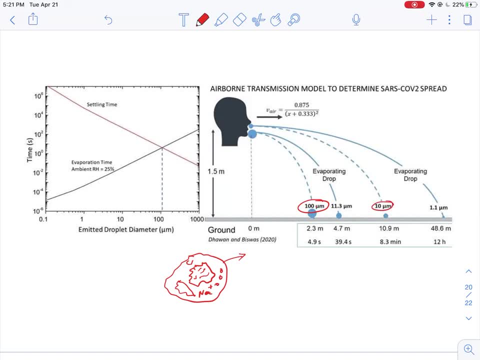 It's possible that they can get shrinked into 10 micrometer or even one micrometer, right. So by having a smaller size, then that means they can stay in the air for a longer time. So Which means that if we cough or if we sneeze, the particles might have a longer lifetime, right. 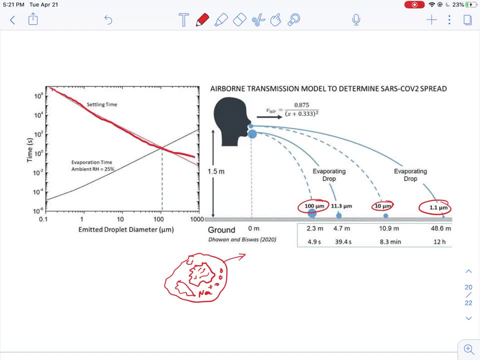 So here it's actually comparing the settling time of particles with different sizes and also the time for the droplet to evaporate. So you can see that basically for particles below 100 micrometer, they're going to have a longer settling time in the air compared to the evaporation time, right? 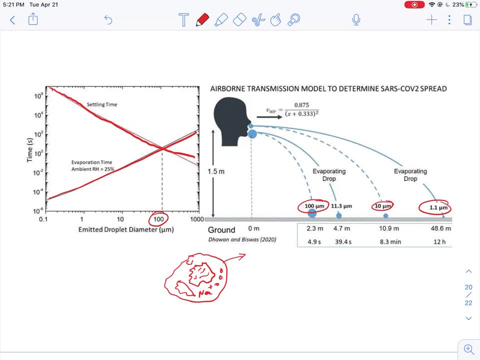 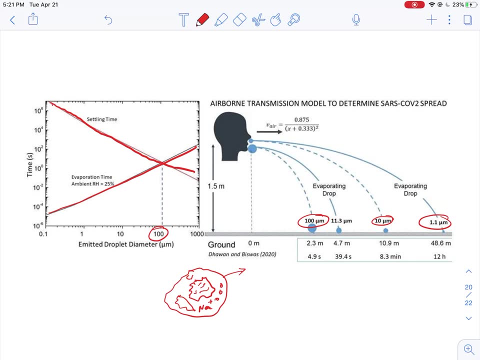 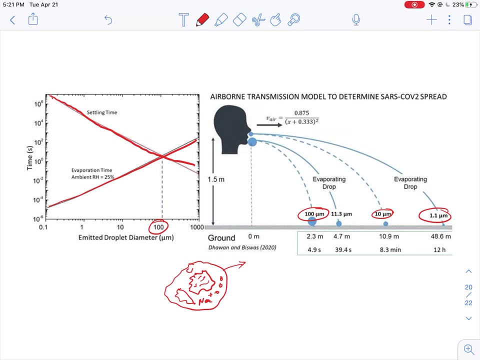 Which means that they're going to be very efficient in staying in the air. So I'm not trying to create a panic situation among all of you, but I would say that the most safe strategy to deal with this virus before we get the vaccines is basically just stay at home, right. 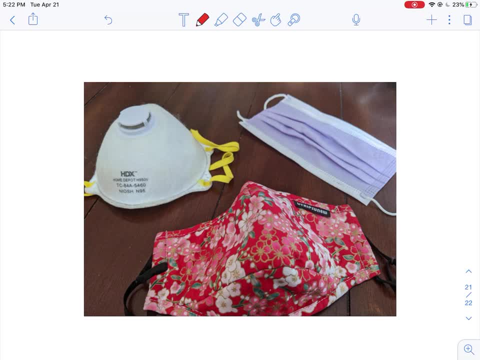 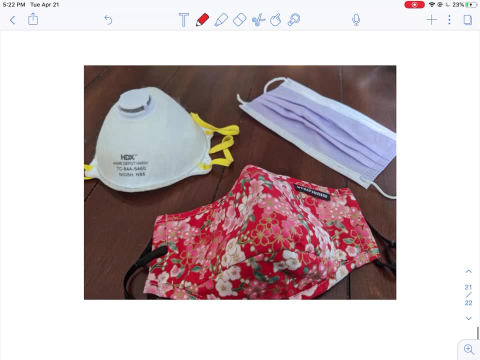 So let's say, if you have to go outside, CDC gives recommendations that we all need to wear masks. right, It's recommended that we all need to wear masks, So there can be different types of masks. We've heard of this N95 mask. 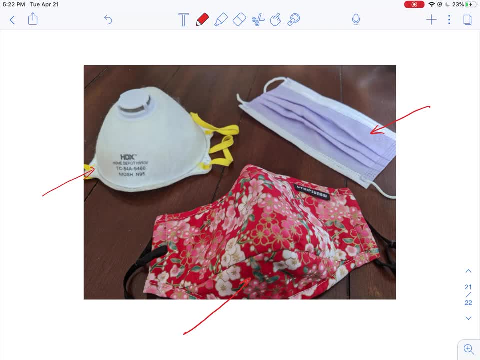 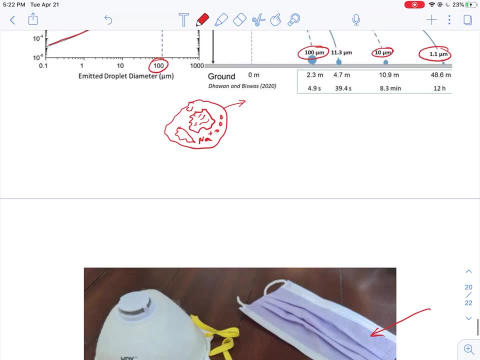 There's also surgical mask, right? So there's also a homemade mask that's made of fabrics. So if you think of how the mask works, so the mask is just a filter, right? So we introduced that we can remove the particles with the filters here. 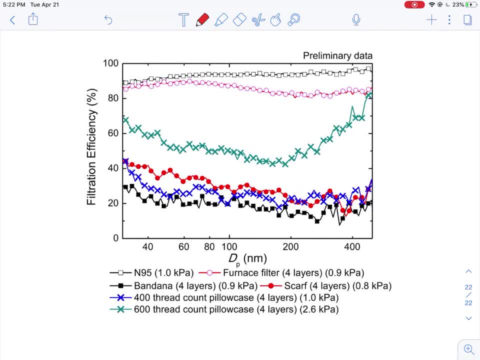 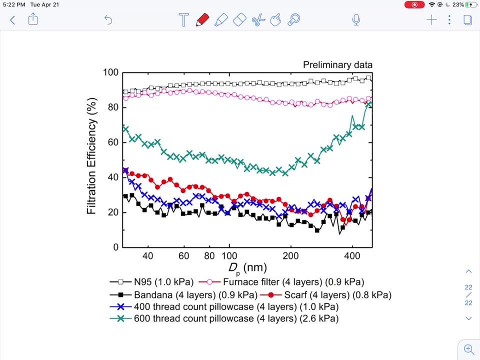 But different filters will have different removal efficiencies. So that's why in our group recently we have been testing a lot of fabrics in terms of its particles. So what you can find out is that for the N95,, which is the most efficient filter for removing the particles, they can have a very high performance efficiency right. 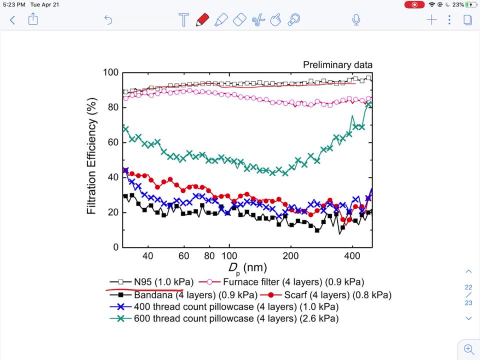 In terms of the filtration. But if you are trying to make your own homemade masks out of fabrics, let's say: if you use bandana, even with four layers, it's not going to give you a high filtration efficiency right. But if you are trying to make your own homemade masks out of fabrics, let's say: if you use bandana, even with four layers, it's not going to give you a high filtration efficiency right.